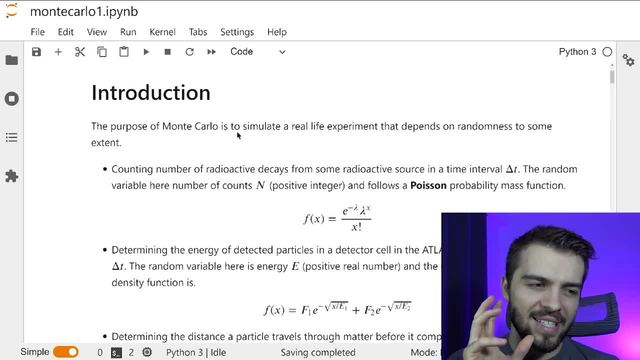 it's useful to give a little bit of an introduction for what exactly Monte Carlo is and what the purpose of it, and so, before we get into any coding, it's useful to give a little bit of an introduction for what exactly Monte Carlo is and what the purpose of it, and so, before we get into any coding, it's 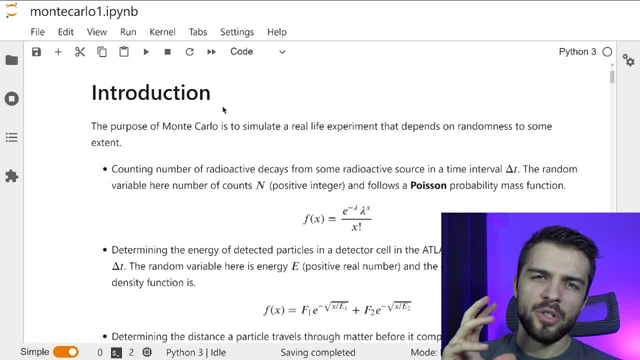 useful to give a little bit of an introduction for what exactly Monte Carlo is and what the purpose of this, and so I would say, and it's defined in slightly different ways depending where you look. so I think the easiest way to express this is as follows: what I have written: 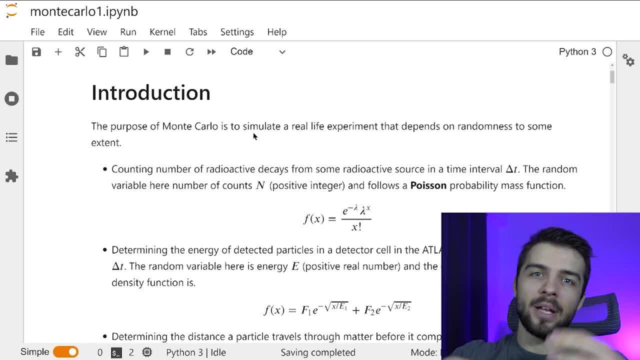 and so I would say- and it's defined in slightly different ways depending where you look to simulate a real-life experiment- that depends on randomness to some extent. so when you do experiments in real life, whether you're, you know, measuring particles in the atlas detector or counting radioactivity from a source, there are elements of randomness that happen in such a thing. 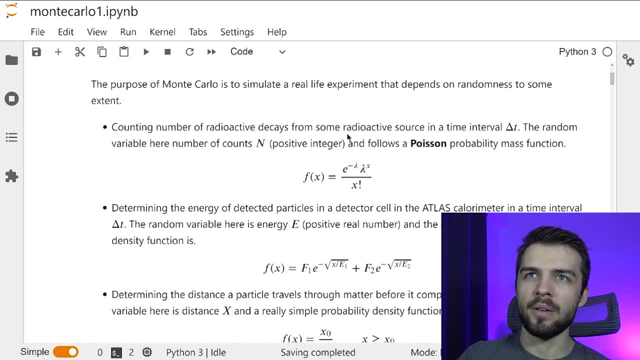 so, for example, like I say here, counting number of radioactive decays from a radioactive source, and suppose you're counting for 10 seconds, well, that's a poisson random variable, and so it has a probability mass function that looks like this. so this is a just a, you know, standard statistics. you. 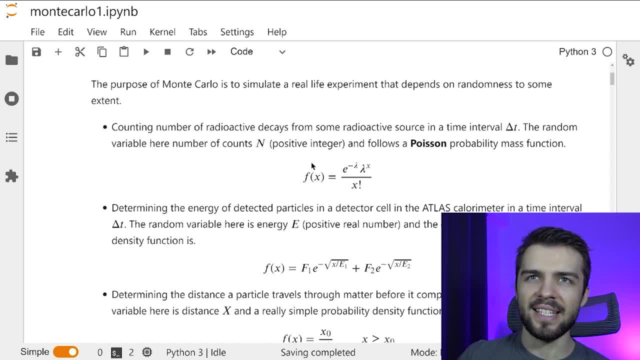 may have seen this before. so if i plug in a value of x, this gives me the probability of that many counts. so if i plug in x equals 1, it'll return a value x equals 2 and lambda is the mean value. lambda doesn't have to be an integer. it could be a you know real number, for example. but i plug in x. 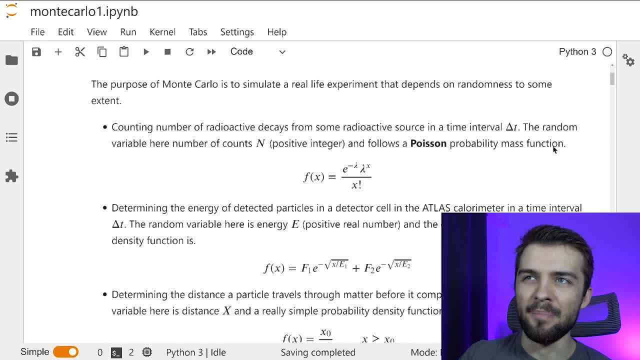 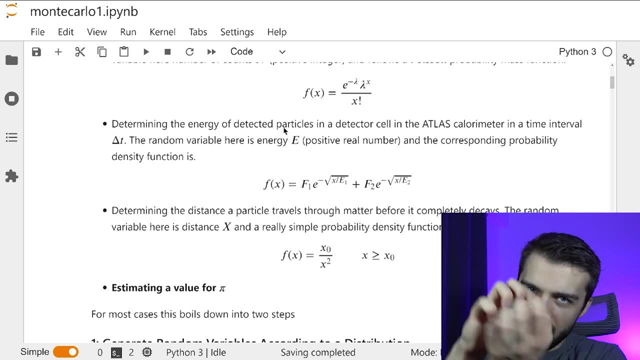 which is an integer here, and it returns for me the probability. that's what a probability mass function does. uh, you know? another experiment: maybe you want to determine the energy of detected particles in a particular detection cell in atlas, which is a huge thing. about what my master's thesis. 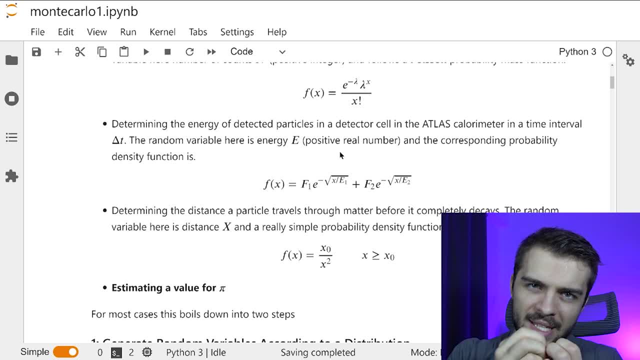 was about, and so here the random variable. the thing that's random isn't the number of counts anymore, like the poisson distribution, but it's the actual energy that's deposited in the cell. so the energy e is the random variable now, and the corresponding probability density function. 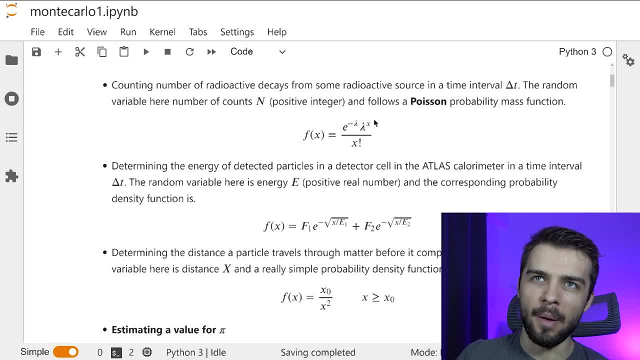 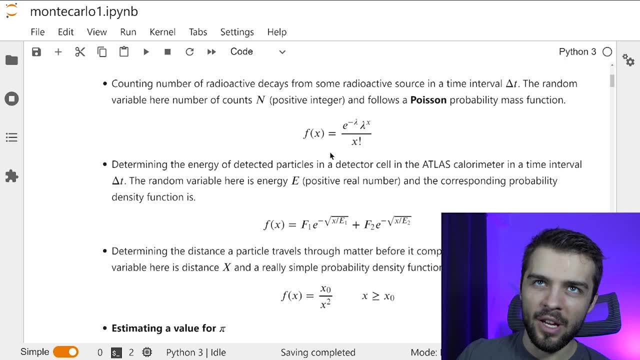 looks like this. so this is different than the probability mass function, the probability mass function. it gives me a direct probability. the probability density function 6x is continuous. here it's not just the number of counts anymore- one, two, three, four, five, six- it's continuous real number. 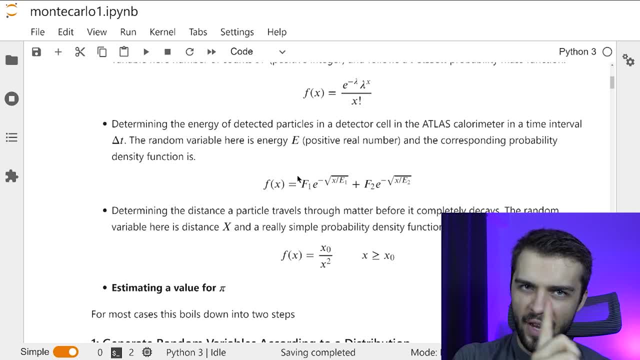 i have to integrate this function between two different values of x and that's how i get the probability, just like a density: if i want the mass, i integrate the density over some space. so if i want the probability, i integrate the probability density function over some region of x. so this is my probability density function here and we'll get into that in. 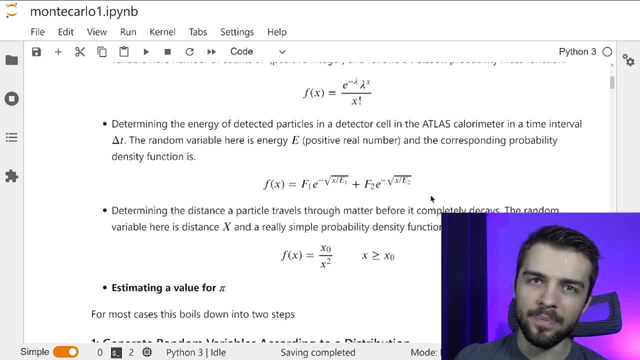 the video. so this is actually a good model for the atlas liquid argon calorimeter. this is a model that i used in my thesis and it represents things really well, and there's particular values of f1, e1, f2 and e2 that you would fit to some real data that you measure. uh, there's another. 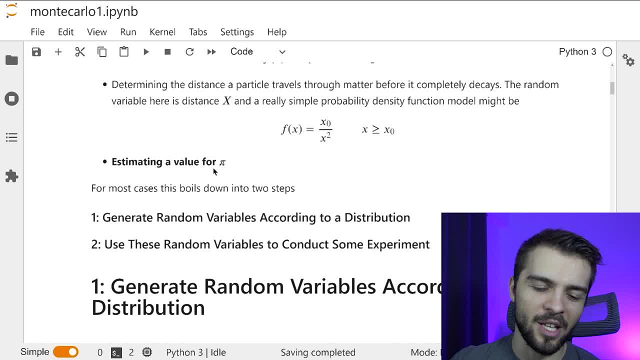 example here you can look at, and then of course, a really famous monte carlo simulation that's really easy to do in python- is you can actually estimate a value for pi. i probably won't do this in this video, but there may be an upcoming video, a short one, where i show how to compute pi really. 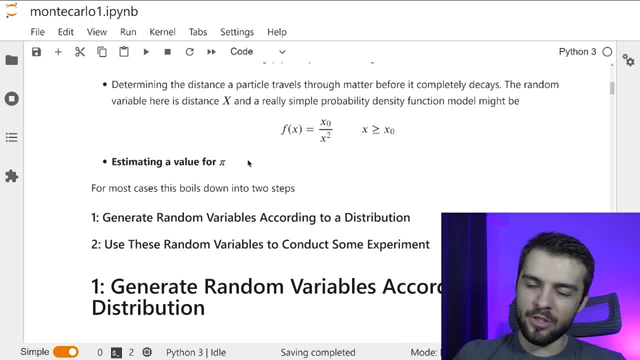 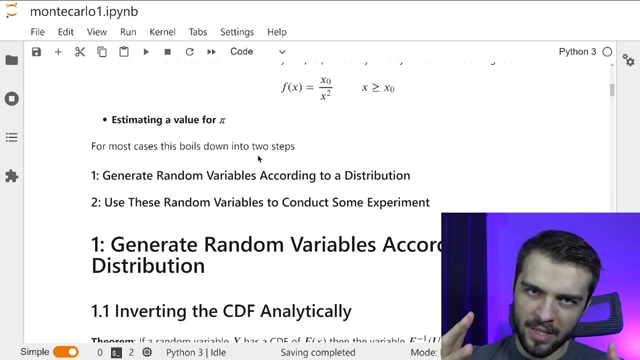 easily in python, because you know pi is an interesting number. as a concept it existed for a long time, but as an actual value- the 3.1418, whatever pi is- that's not so trivial to come up with. so for most cases when you're simulating an experiment, there's two essential steps here. 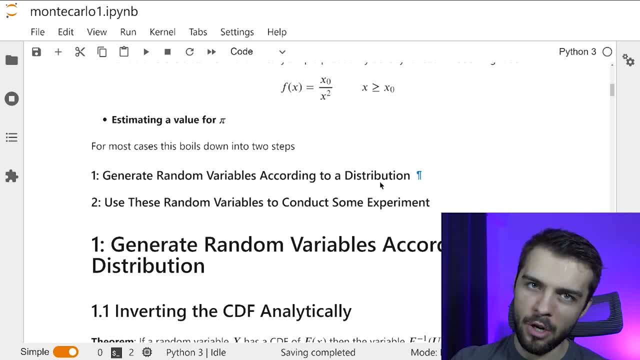 you want to generate random variables according to a distribution. you know, maybe a poisson variable could be a variable that's looks like this or any other thing that you know is relevant to your experiment- and you want to use these random variables to conduct some sort of 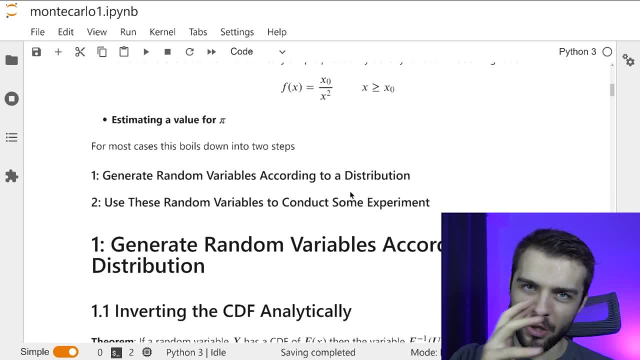 experiment, and that's sort of vague how I've said it right now, but I'll sort of go through one and two and I'll go through everything and I'll show you how this is sort of done. so the first step, and all these things, is to actually 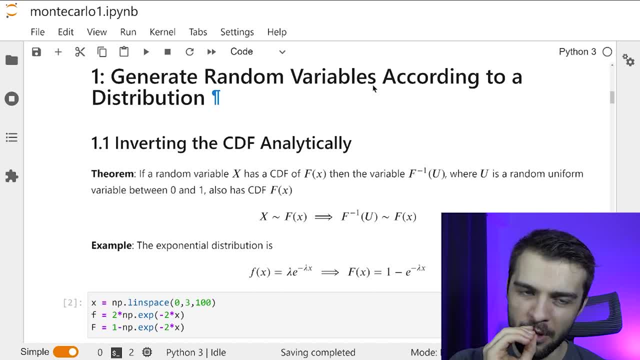 generate random variables according to a specific distribution, and that's not as easy as it always sounds right. I mean, you know that computers can generate random numbers. they can generate random uniform numbers and if you have a package like numpy I can generate lots of different types of random numbers. but 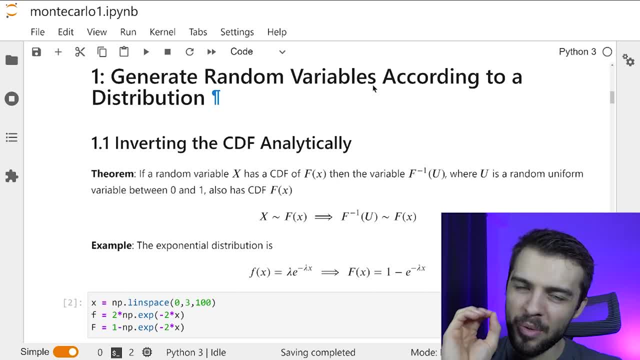 suppose you have a distribution that's not in numpy, how would you actually generate a random number according to a distribution? and there's a really useful theorem here- and this is the most important theorem, I think, for Monte Carlo, and it's really useful to sit, read it and really understand it. so it goes. 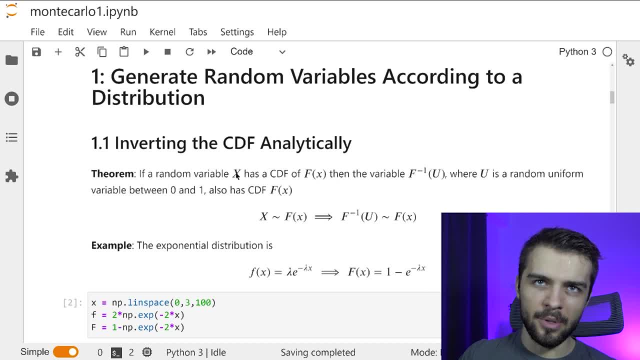 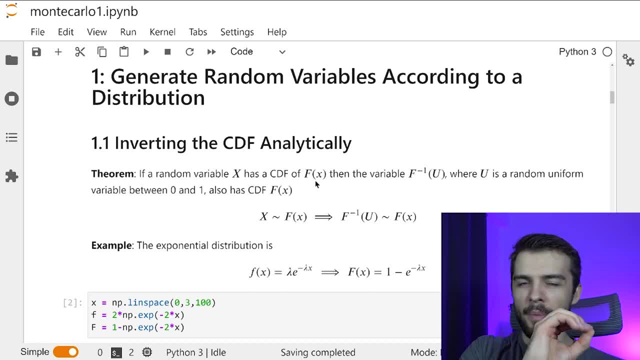 down to the í cakes, up to the root qui-caps A and Y, going up to the left and up all the way up to the right, so the X can generate a really simple distribution. so if you know the function f of X, that's ninja, that's a. 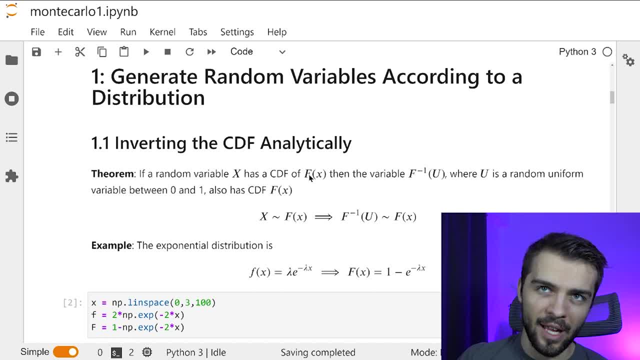 cumulative density function f of X. that's useful to know what that is. the C, D, F. so the probability integral from negative infinity to X of the probability density function in the case of simple distributions. so if X has a CDF of F, that's unique. if you know little f, you know Big F. 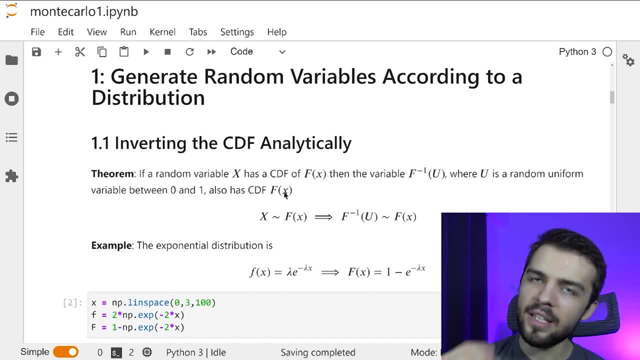 also has cdf, f of x. so that's a lot and i've written it really simply here. so x, this means distributed according to f of x. that implies that f inverse of u, where this is a random number uniform between zero and one, also has this distribution. so this x and this both have the 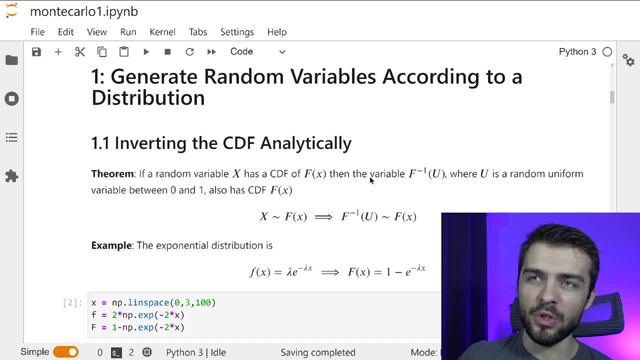 same distribution. so that's a really useful tool. if i can generate lots of u's, a lot of numbers between zero and one, and i plug them into f inverse and i compute numbers, they'll be distributed the same as x. so this is the key result that sort of all monte carlo is based on to some extent. so 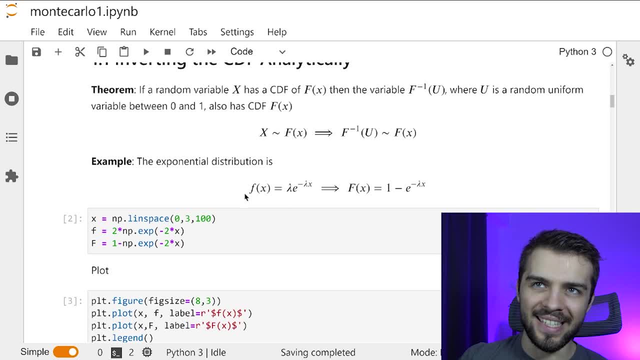 for example, let's look at the exponential distribution here: the, the probability density function, is equal to lambda e, the negative lambda x. the cumulative density function, which is the integral of this from negative infinity to x, is one minus e to the negative lambda x. so this is: 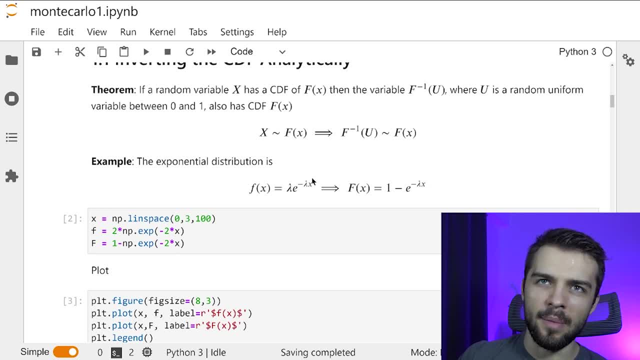 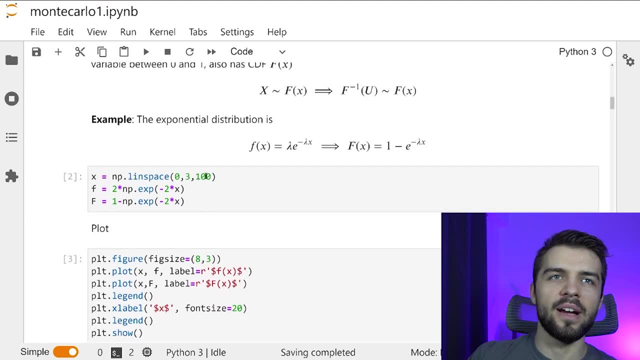 what capital f of x is, suppose i want to generate random numbers according to this distribution. well, we can do that. and before we do that, let's actually look at f, little f and big f. so here i make some x variables from zero to three to hundred. let's import the packages here. 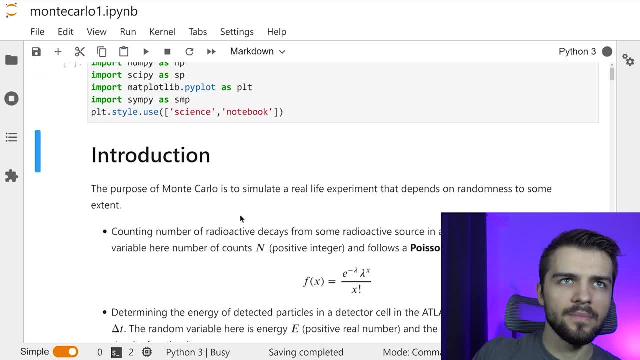 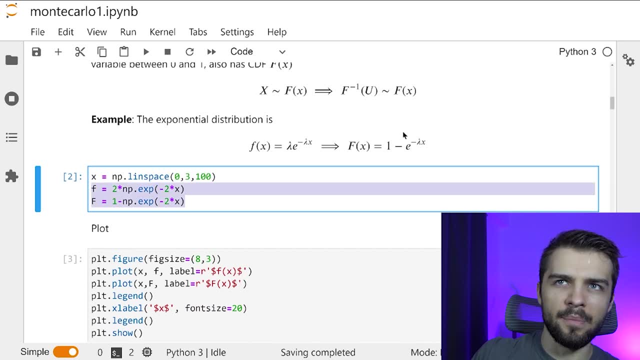 so here i just make a hundred things between zero and three, and i'm just plugging in little f and big f, and here lambda is equal to two. so let's actually plot these functions right. so i'm just going to plug in little f and big f, and here lambda is equal to two. 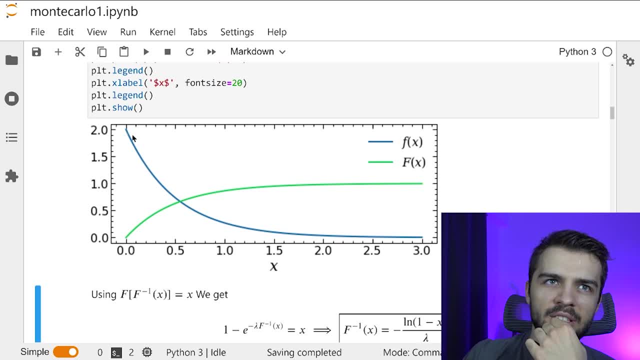 right. so i'm just going to plug in little f and big f, and here lambda is equal to two, and so i have x and f and x and big f, and you can see that little f of x it looks like this: there's more probability of um, you know, whatever being in this region, of x being here, and then 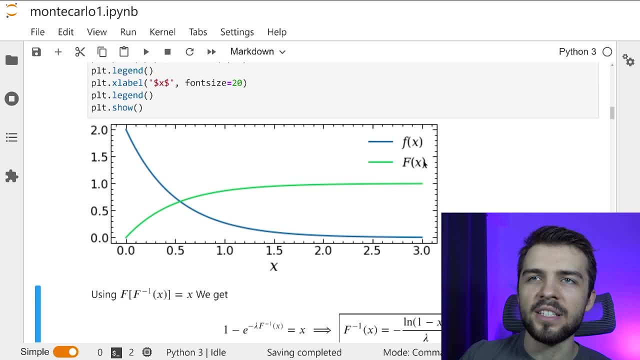 less of it being here. and then capital f of x, which is the cumulative density function. it goes between zero and one, it's like a hundred percent. so if i go here, this is the probability that you know, the random variable is less than or equal to this value. so if i'm way out here and 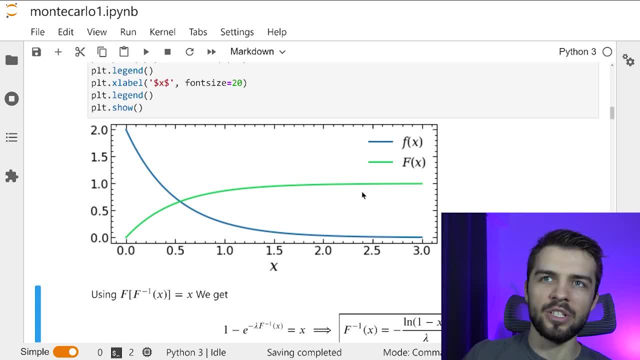 it's one. you're basically a hundred percent that it's somewhere in this region, less than that number. that's what the cumulative density function is. so i'm just going to plot these. so i'm just going to plot these. the word cumulative right cumulative density function says so. these are what these functions. 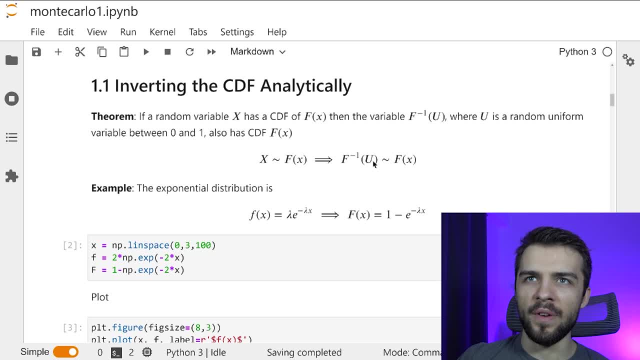 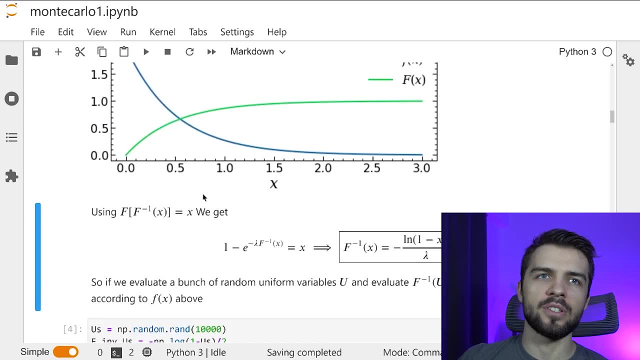 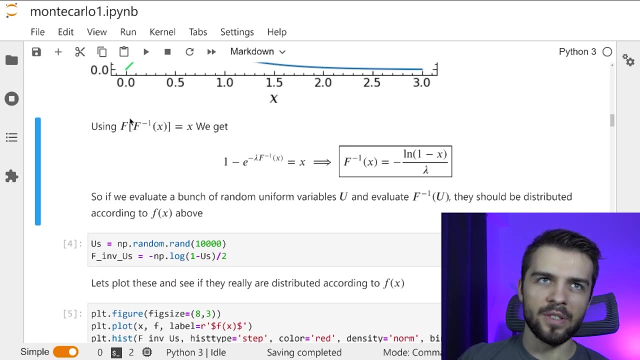 look like now. in order to compute f inverse of u, which is going to give us our random exponential variables, we have to compute f inverse. so you know there's a simple way of doing that with math. i use f of f. inverse of x equals x. that's the identity here. then i plug f inverse. 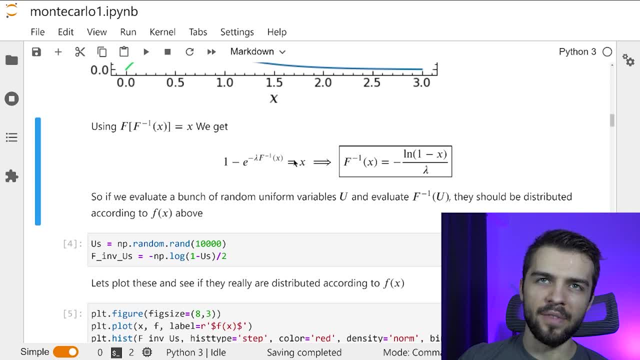 of x into capital f. so one minus e to the negative lambda f inverse of x equals x. that's just this formula here. but plugging in the negative lambda f inverse of x equals x. that's the identity here. but plugging in what i know capital f is equal to. so this is useful for that, and then i solve for. 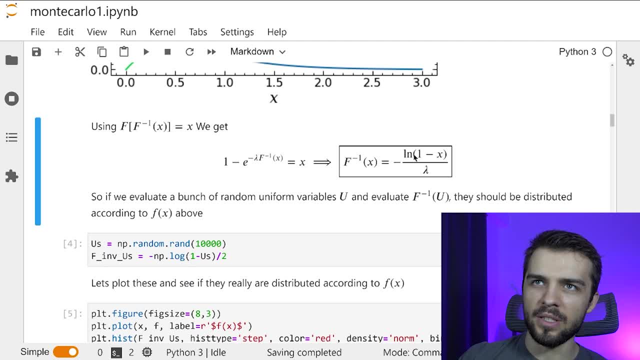 capital, f inverse of x. and i get this formula: f inverse of x equals minus ln, one minus x over lambda. so this is what the inverse function looks like. so if i generate a bunch of u's and i plug them in here, what the theorem says is that they're going to be distributed according to an exponential. 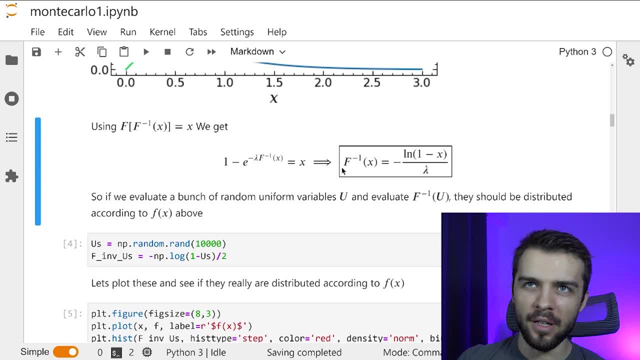 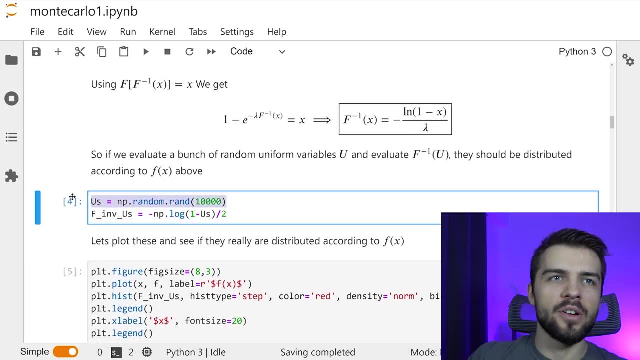 distribution, right. so i'm going to make a bunch of u's, i'm going to plug them into this function, this weird looking function here, and they're going to be distributed exactly the same way. so that's what i do here. so here i'm generating uh, ten thousand random, uh, uniform variables between: 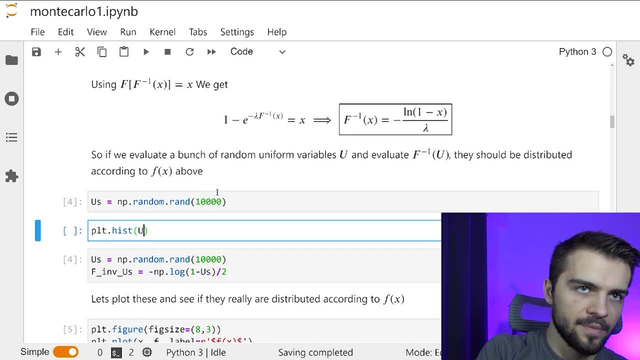 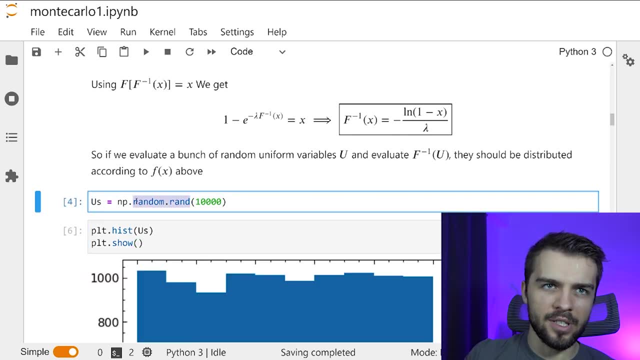 zero and one and i can make a histogram of them just to prove this to you and let's show this here. you can see that these u's, these are random uniform. that's how i call this in numpy and it's about uniform between zero and one. you can see that they're distributed like this. so that's sort. 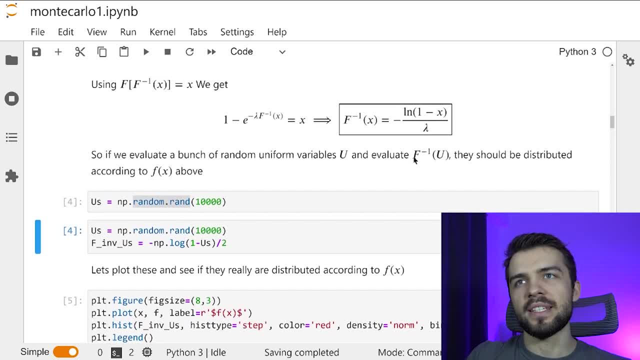 of exactly what we want and we're going to use those to generate these capital f inverse of u's to get exponential distribution variables. so i call this my f inverse u's, which is plugging in u to this function, and i just plug in all these values of u's into this function here. so i evaluate them and now i'm 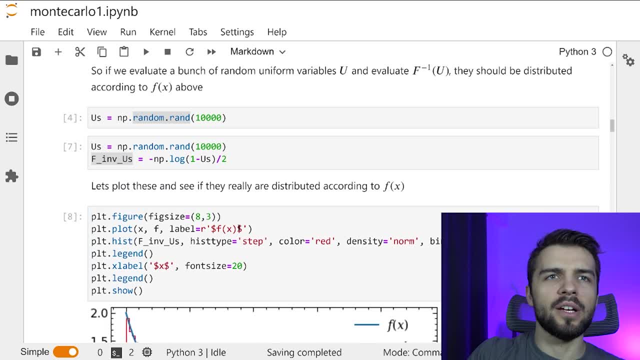 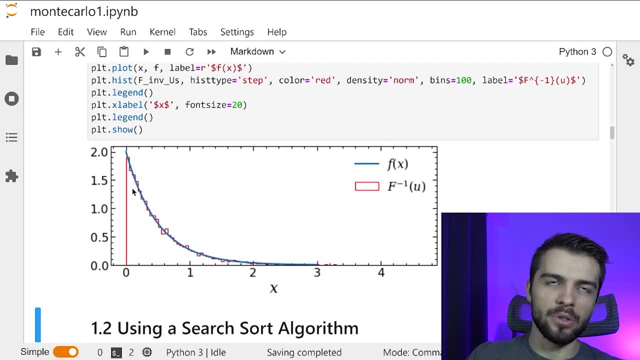 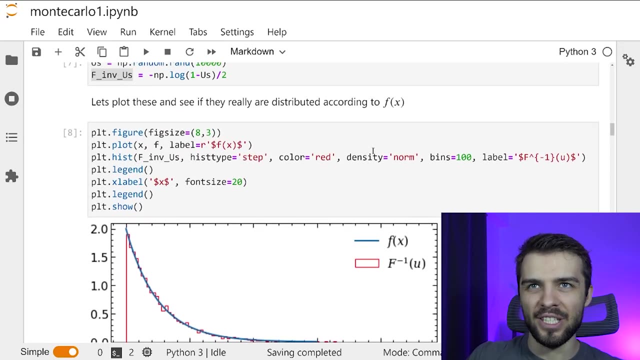 going to make a histogram of this f inverse of u's. so what i do here is i'm looking at. so first two things. there's the probability density function, here f blue. i showed that above here as well and you can see that i have a histogram of these random variables and i've normalized the histogram. 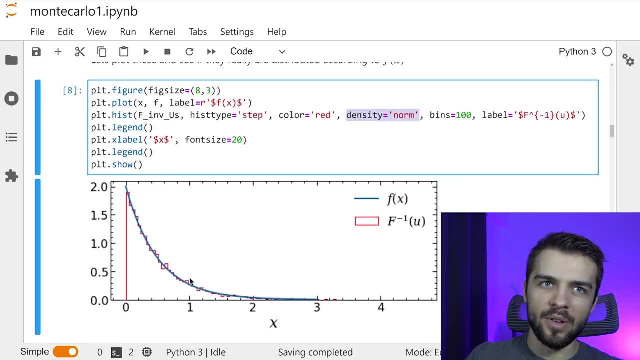 here about friesi for thisaren's number of év of day. this is the name of the Williamians theorem here and this is shown here. that, oh, that is a number okay for rows. the return time that i might modify theashi for this cu pawn is多少 prime of the value of x, emperor, and then what i? 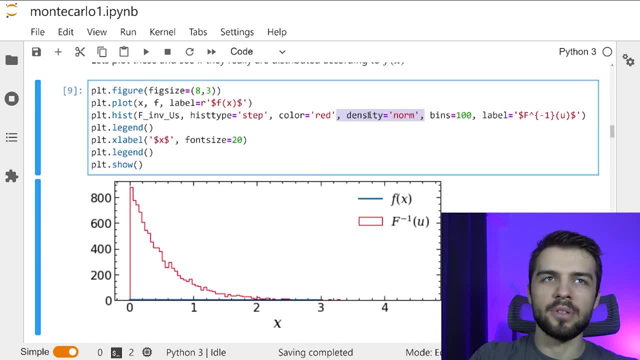 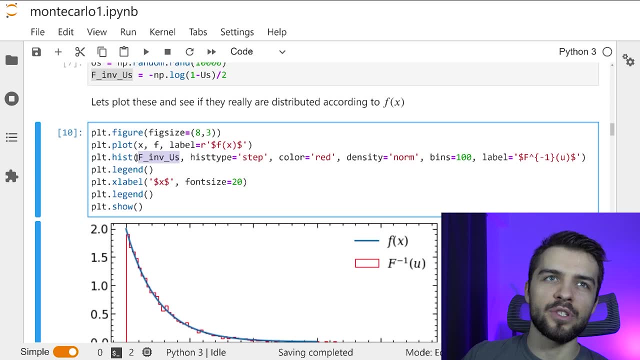 mean by this is that i want the probability density in order of this, you can see that the probability density equals norm, so that the area under the histogram equals one, just like how the area under f of x equals one. if i didn't have this here, for example, if i deleted this, 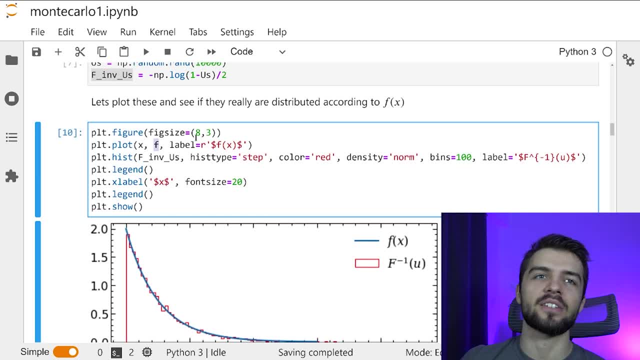 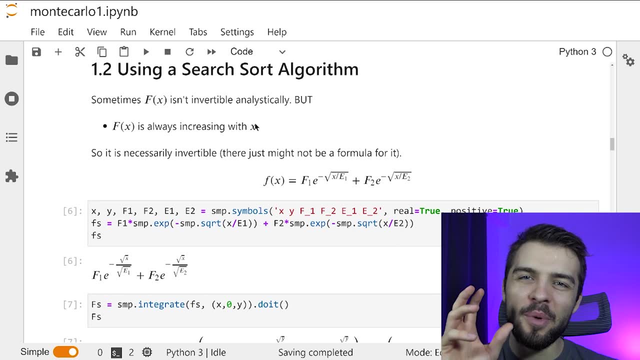 f of x right and have a cdf capital f of x. you can see that it follows it exactly. So I have a really good method now for generating random variables. So there's a little bit of a fly in the ointment, and I'm sure you've maybe thought about this when I was going through the previous 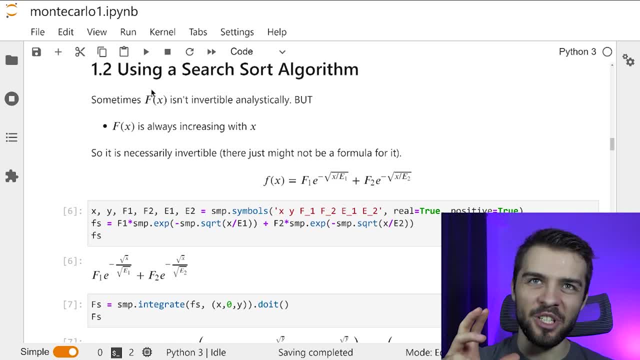 step. Well, what if capital f of x isn't actually invertible? What if there is no f inverse of x? Well, let's think about that for a sec, because we know that capital f of x is always increasing with x, right? If I look at this plot here, I know that the probability of being less than or 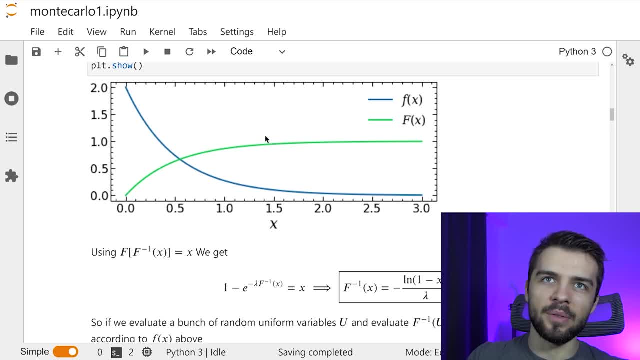 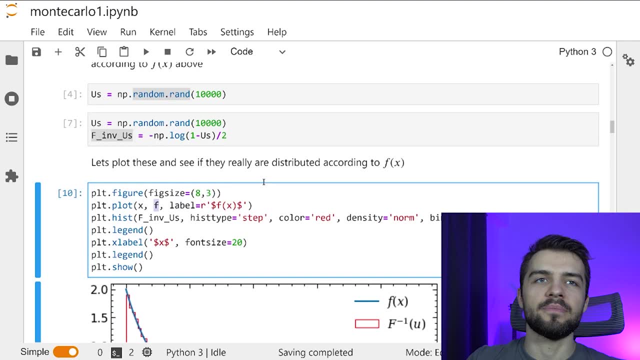 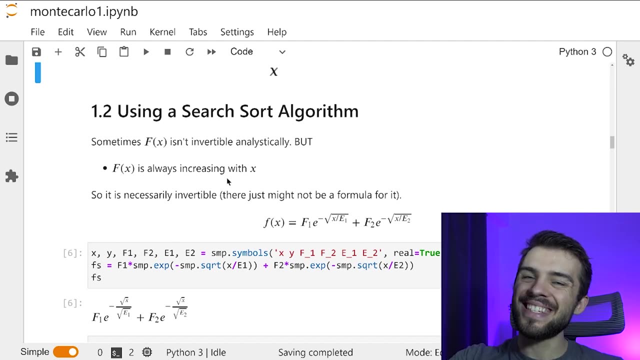 equal to this is going to be greater than the probability of less than or equal to this, just because I have more stuff right. So capital f of x is always increasing. This is true for every distribution right, And so if capital f is always increasing, there's necessarily an inverse. 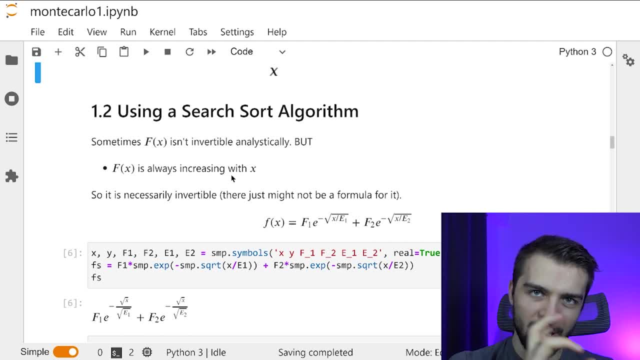 It doesn't mean that there's an analytical inverse like a formula that we can actually solve for, but it is necessarily invertible, Right, Unless of course it's constant and then maybe you have a discontinuity, but it's. 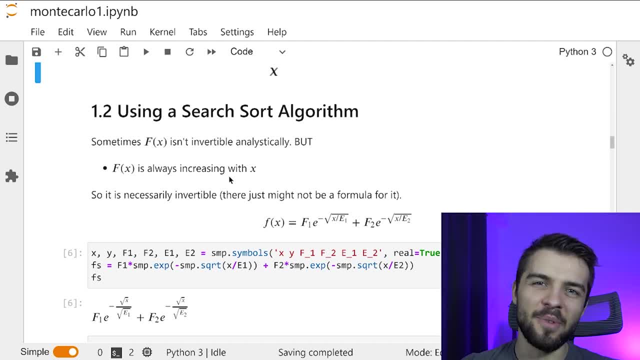 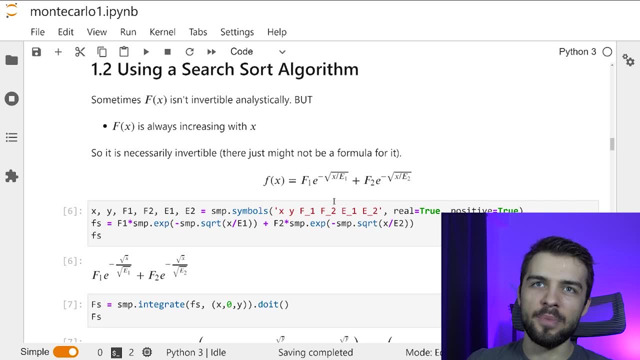 basically invertible is what I would say. A mathematician might get mad at me for saying that, but you know it's basically invertible. And so, for example, look at this formula here: This was the distribution of energy in an atlas calorimeter cell, for example. So it looks like this: So 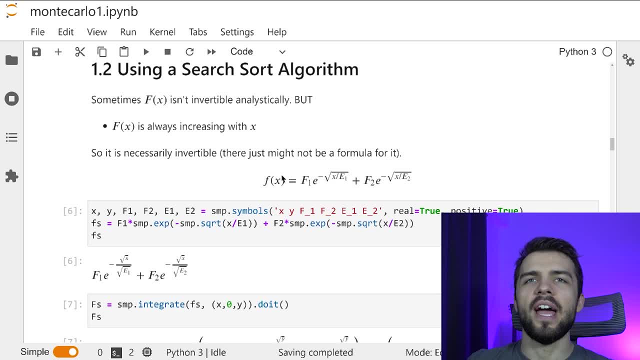 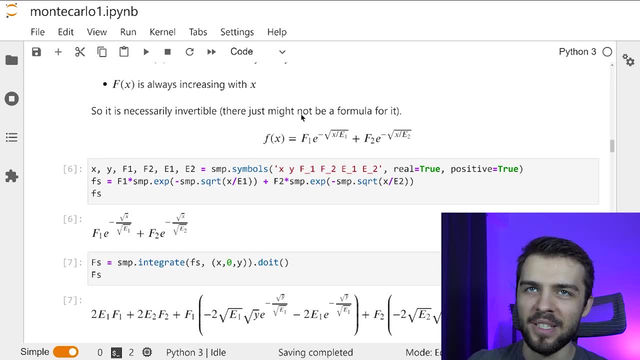 let's actually plot this distribution before I get into the example and the cumulative distribution as well. So here I'm using SymPy to actually come up with the formula. for the formula, I want to find the CDF, which means I have to find the integral of this And rather than 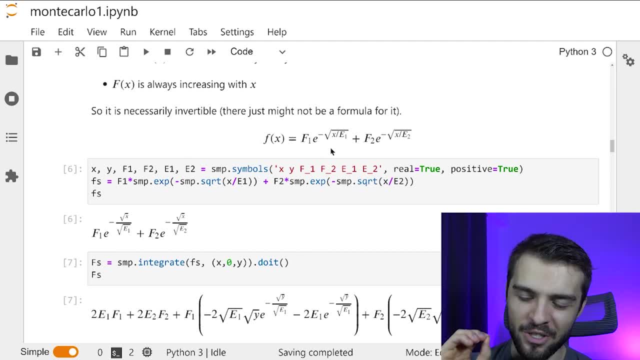 do it by hand or show you a bunch of mathematical steps. I'm just going to do it in SymPy and show you the power of SymPy, as I always do So. here I define x and y and then the four variables here 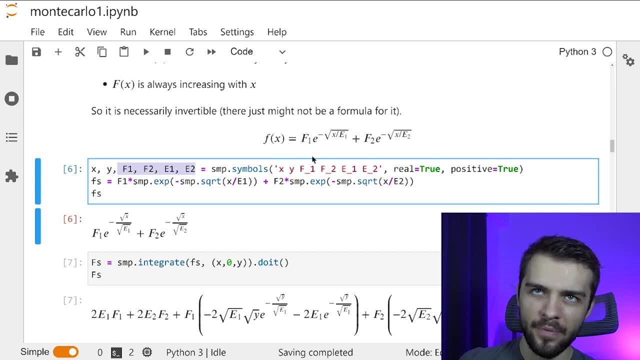 f1, f2,, e1, and e2.. They're both real and positive for this distribution. here, And I define my f and s stands for symbolic, So if you see an s after a variable, it means I'm dealing with a. 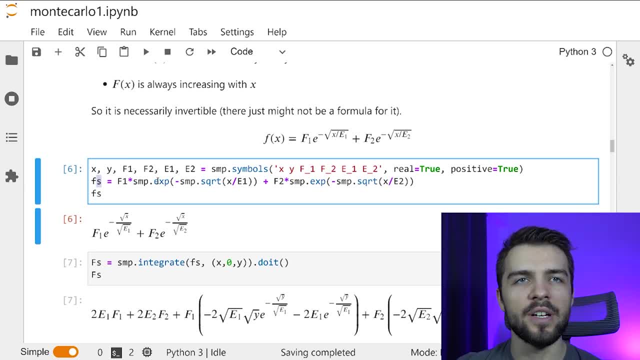 symbolic thing. So my symbolic function looks like this. So I'm going to define my f and s stands for this f1 times symph of this. It's just this formula in SymPy And I can look at it and I 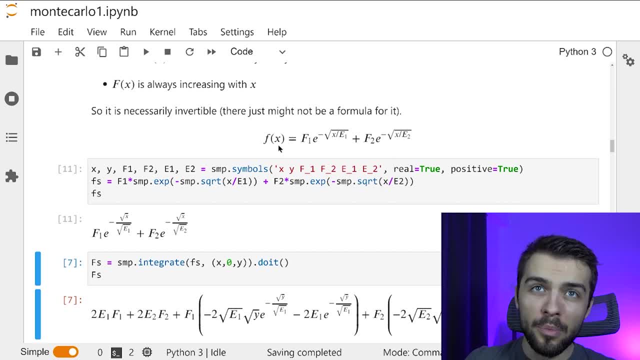 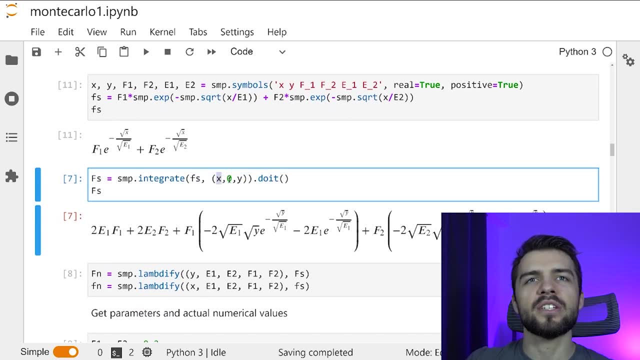 truly do get this formula. And if I want the cumulative distribution function, well, what do I need to do? I need to integrate this function here, which is f symbolic, And I want to integrate x from 0 to y. Now you might be wondering: why am I going 0 to y? Well, I can't use x twice, right? 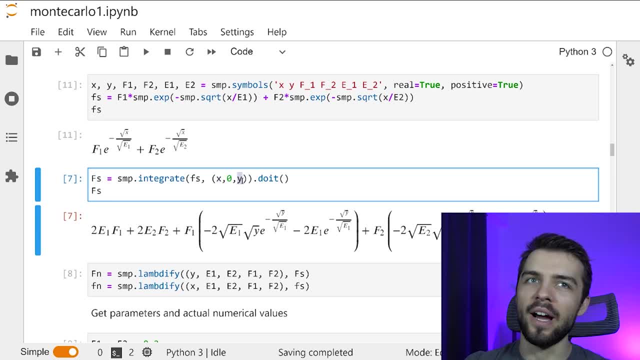 So I'm going to go from 0 to some other variable that I'm going to call y. So I integrate my symbolic probability density function to get the cumulative distribution And I'm going to go from 0 to 0. And I'm going to take my cumulative function using SymPy. I call this And then 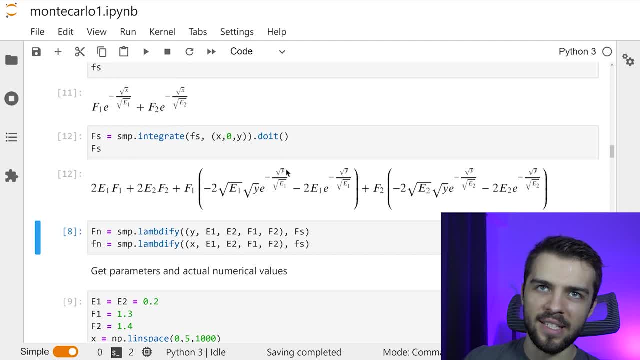 lo and behold, I get my cumulative density function with y instead of x here, But it's really the same thing. y is the variable that's interesting here, So it's a big long function. Now the issue is right. we want to make compute f inverse here, But I don't really feel like. 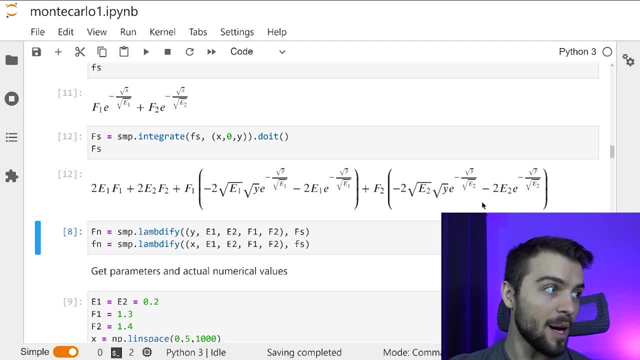 taking the inverse of this function. I don't know if there really is an inverse- There might be not, as far as I know- to this function here, And so what we want to do is we want to find another way to take the inverse of this function, sort of using a computer, And I'll show you the. 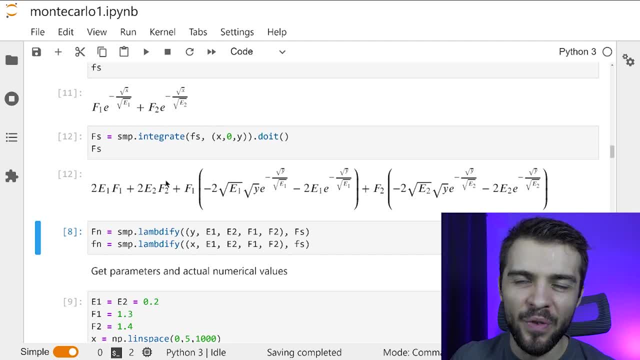 sort of trick here. So the first thing we'll do is we'll convert this function here to a numerical Python function. So that's n here. Whenever you see an n, that means a numerical function. It means I give it numbers and it returns a number. in Python It's a normal function To do that. 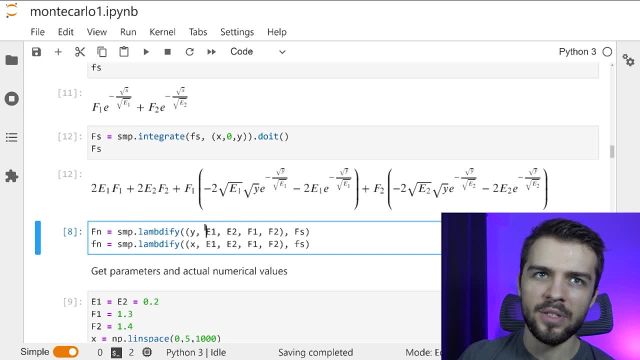 I have to lambdify the symbolic function. You've seen this in my other videos. These are the input arguments. This is the symbolic expression here And this will turn it into a numerical function where I can actually give it arguments. So I can run that Here I have. 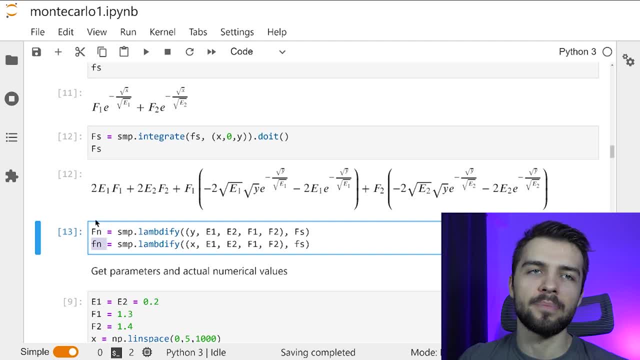 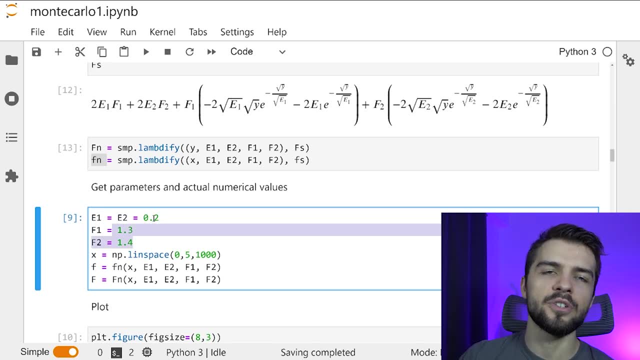 a numerical function for the cumulative distribution function and the regular probability density function. So I give it some sort of numbers here. e1 and e2 are equal- and then two different values of f1 and f2.. And I'll plot it between 0 and 5.. And so here I'm actually obtaining values. There's. 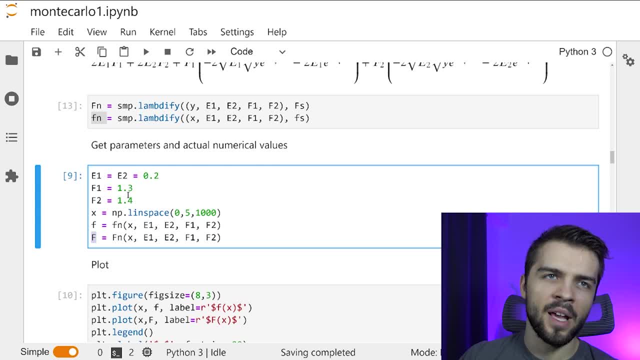 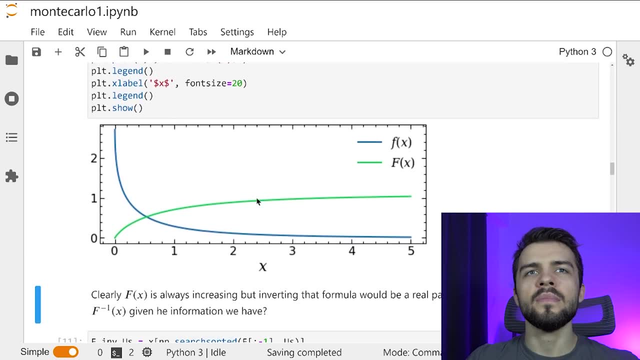 no, n or s. These are actual values for f and capital F. So I'm going to plot this function. I'm going to plot both the density function and the cumulative function here of these two functions. So you can see little f of x. the distribution looks like this. So there's a lot more chance of 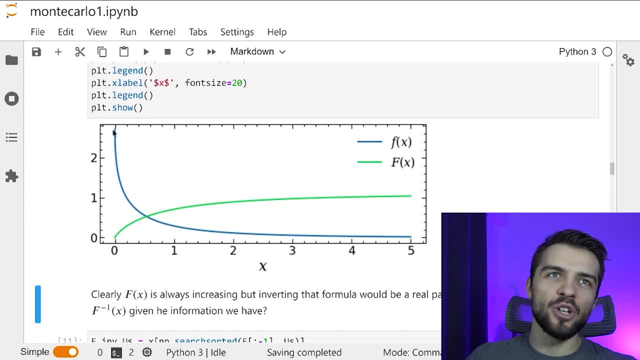 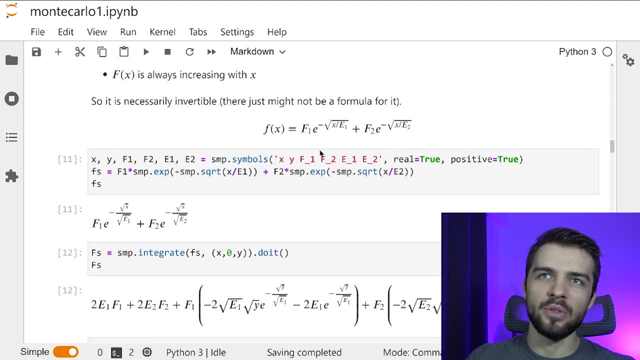 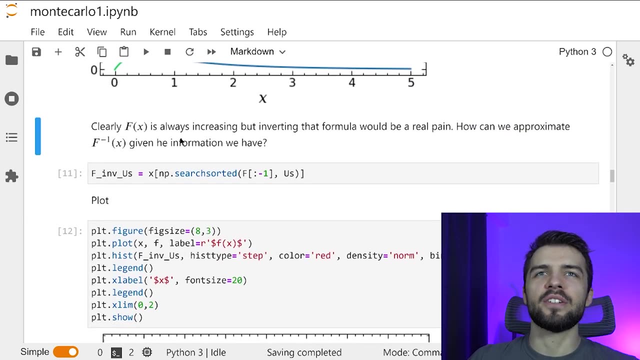 getting lower energy and then less chance of higher energy, And it's not quite exponentially decaying, It's sort of decaying in this square root exponential fashion, with two different terms here. So, like I said, clearly, capital F of x is always increasing. right, You can see it's. 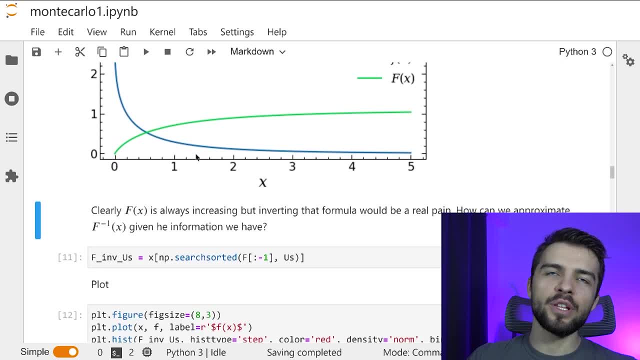 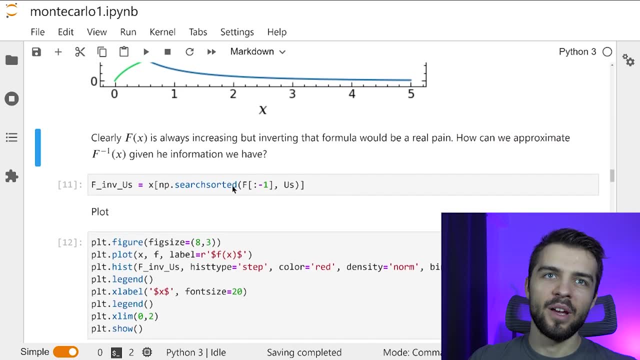 always increasing, like I said it would for most distributions. But inverting the formula is really hard, And so how can we approximate f inverse of x, given the information that we have? Well, it turns out you can do it in this one line here, And you know, that's obviously really fast, and 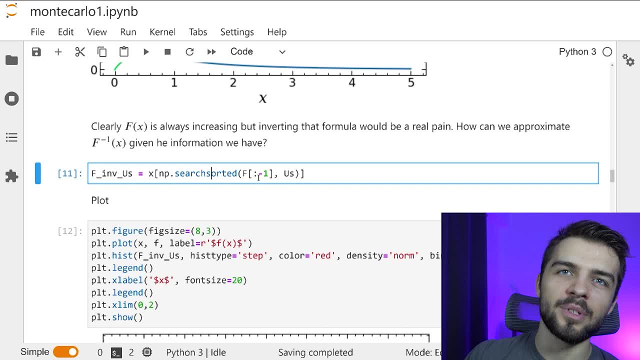 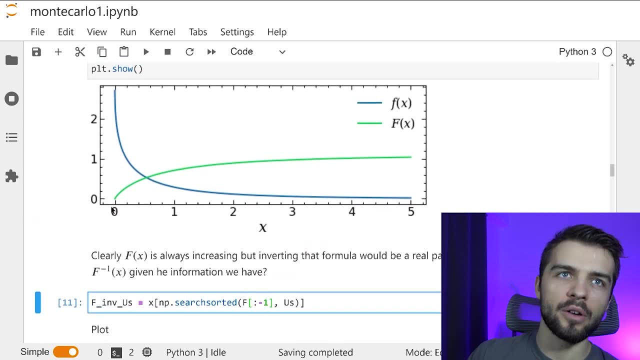 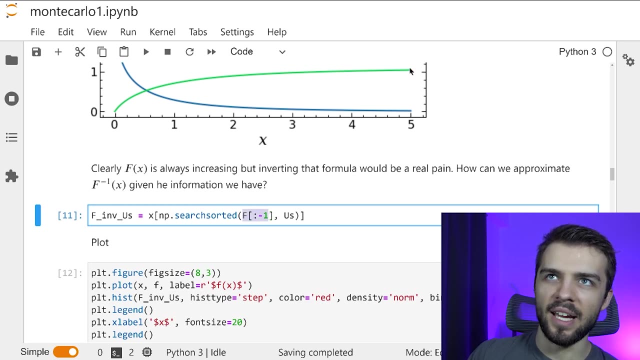 I'll explain it. But here's what we do, And this is essentially what's going on here. So I take my capital F and I go from the- so the literal numerical values that I've plotted here, right, That's what the capital F array is- And I go from the first point to the- you know, second, last. 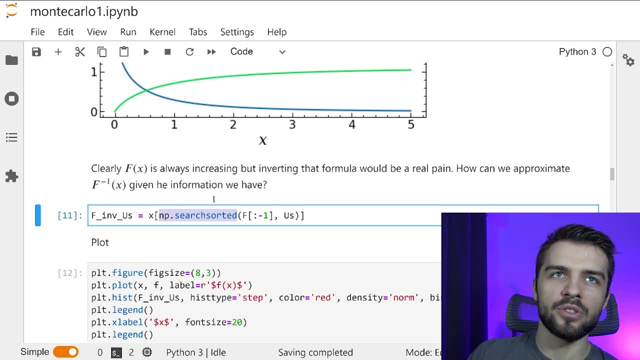 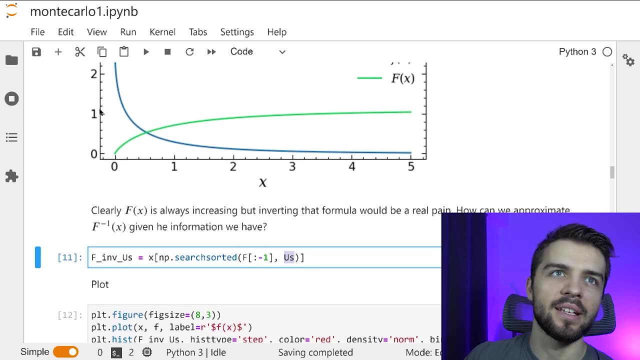 one right, And I call this npsearchSorted on this array of all these values and all my random uniform numbers as well that I've generated. And so what that does is it says: okay, well, I know the user between zero and one right, So they're sort of here like this: And so I have u. 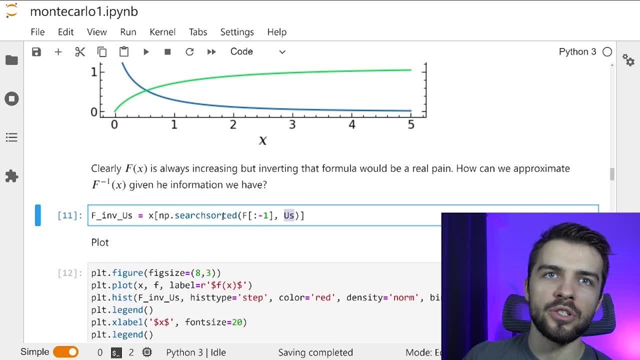 is equal to 0.2,, for example. What npsearchSorted will do is it'll look at this array of f values and it'll give me the index. So not the x value, but the index, this array where the u's would fit in between to keep this sorted. So what it means is that 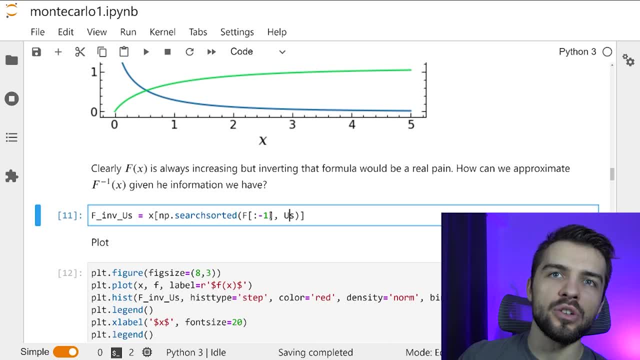 it'll essentially find the index where, if I were to insert this value of u, maybe 0.2, into this array, given that this is always increasing, what would be the index I would have to insert it into to keep that array indexing. So if I had like 0.1,, 0.3,, 0.7,, 0.9, and I was giving a value, 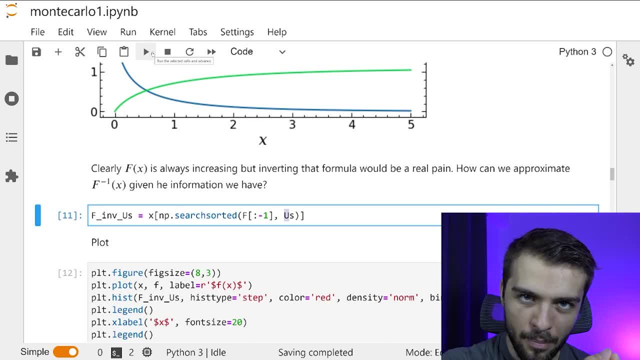 of u, I would have to insert it into the index. So if I had like 0.1,, 0.3,, 0.7,, 0.9, and I was giving a value of 0.4, I know that 0.4 would have to come after 0.3 and before 0.7, right, And that's. 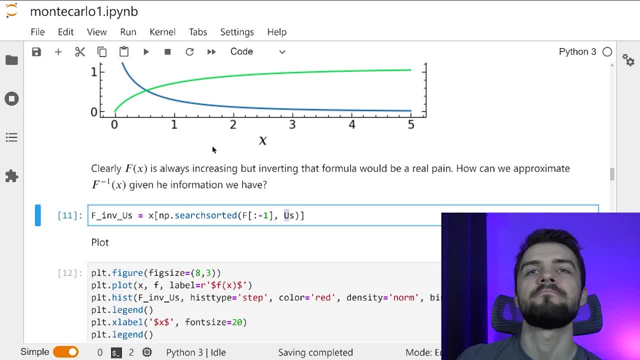 the index. So I would find the index of that, and that's the index it would return, And so that's what's going on here. So it gives the indexes here, And if I want the x value, I just call x, and this would be an array of indices, right? And so it'll give me the x values at all these. 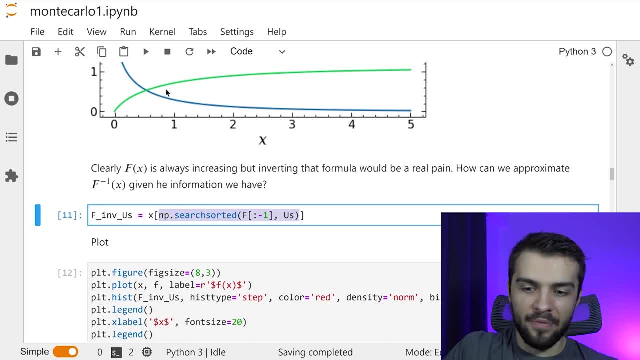 different indices here, And then I have the x's that I want. right? This is what the inverse function is. It says: give me the x value such that this is the y value. So if it's like 0.6 here, it's saying: 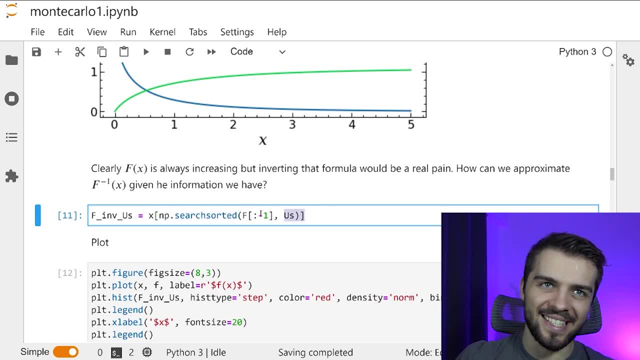 give me the x value such that y is equal to 0.6.. That's what this essentially does here. So again, if you're still confused, I'd recommend looking at what npsearch sorted actually does. But this is computing the inverse function. It says: give me the x value such that 0.2 is the y value. 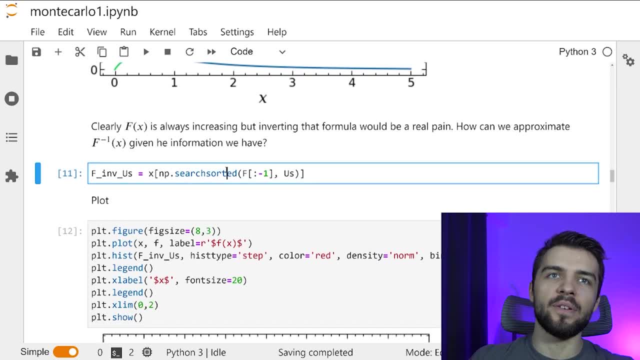 right, And that's sort of what's going on here. So I can compute my f inverse of u's in this way. This is the numerical way of doing this And I can plot them just to make sure that it is indeed that these values are distributed according to little f, which is the probability density. 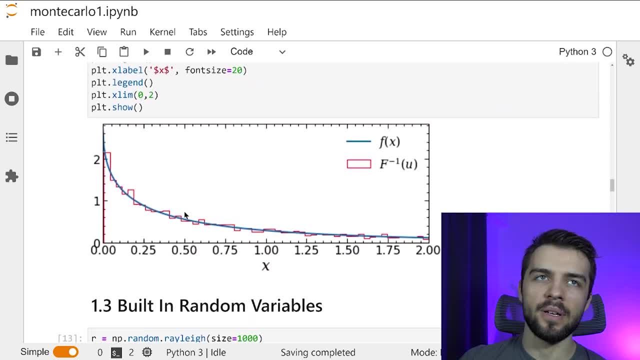 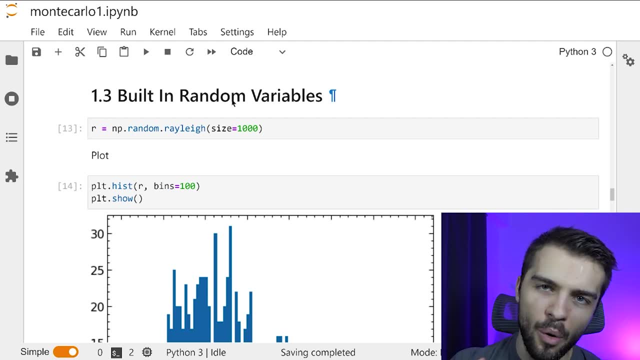 function And you can see, indeed, that they are they sort of match up here. So the thing that we did worked really well. So finally, of course, there's built in random variables in NumPy, Like you don't always have to do this thing every time you want to generate a certain type of random. 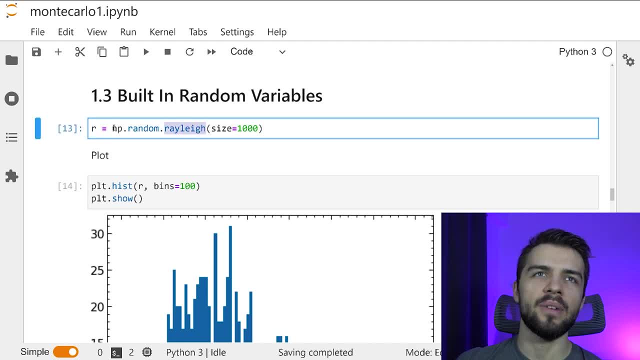 variable. So here I'm looking at the Rayleigh distribution. It's a particular probability distribution and there's tons of others in NumPy as well, And so here I can generate a bunch of random numbers and I can plot them And you can see. 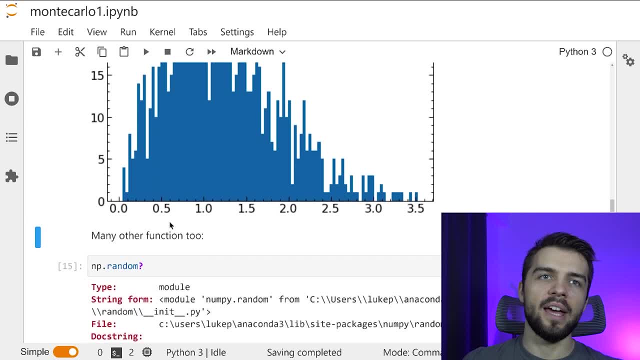 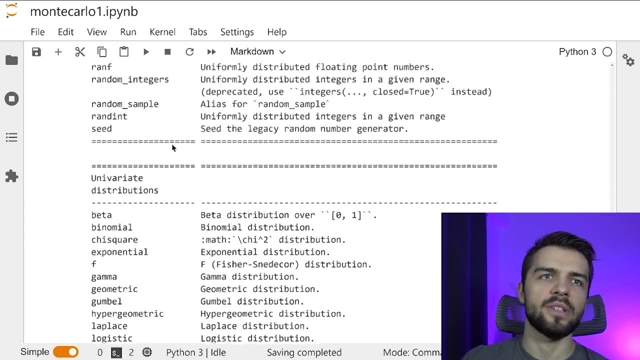 that they're distributed according to a certain distribution here And there's lots of other functions in NumPyrandom And so we can actually look here at all the different types of functions And you can see if I scroll down. we got beta distribution: binomial chi-squared exponential. 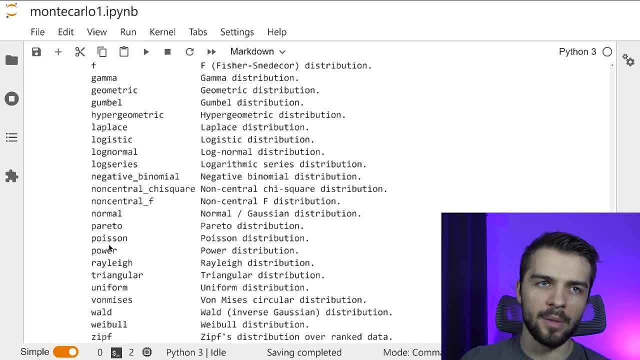 Fisher, distribution, gamma, geometric. So all of these are available to you. So if you're doing a particular type of random variable, definitely make sure that it's in Python and NumPy first, before you go and try to invert a cumulative distribution function and generate things that. 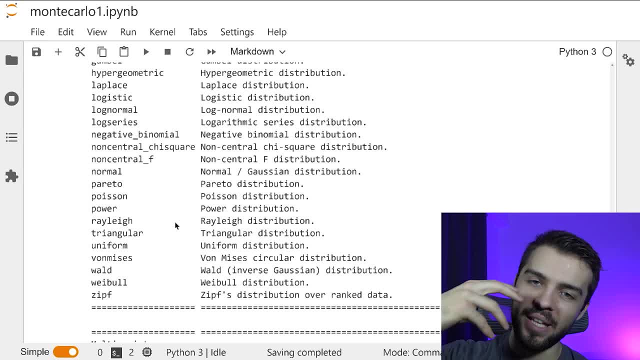 way. So there are lots of built in functions and then even probably extensions of these and other packages in Python as well. So before you do the other steps that I did, unless you have your own distribution, that's a little bit unique- look to make sure it's in NumPy And then you can just 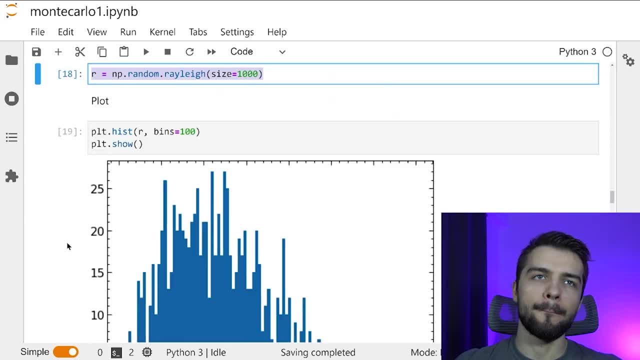 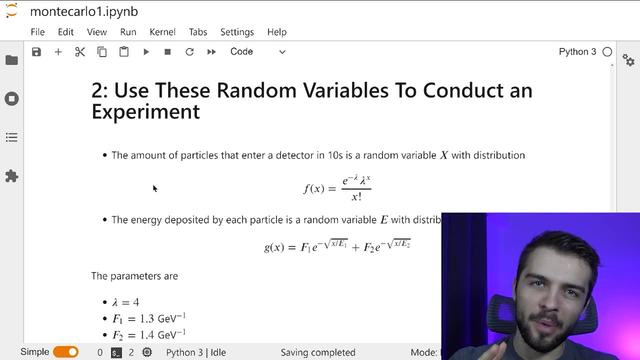 generate a bunch of random numbers like this And then you can generate a bunch of random numbers in a one liner. So now we get to part two, and that's actually using these random variables to conduct an experiment. And I sort of left that a little bit vague before And I'll go over an 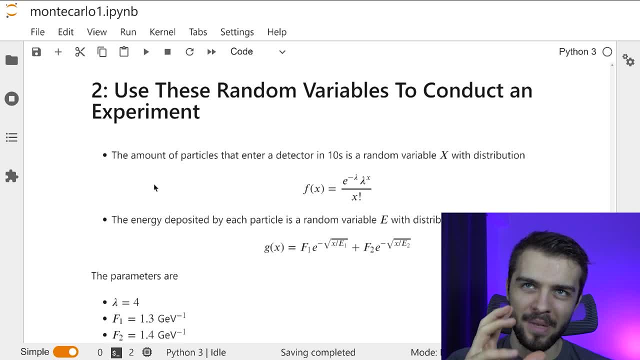 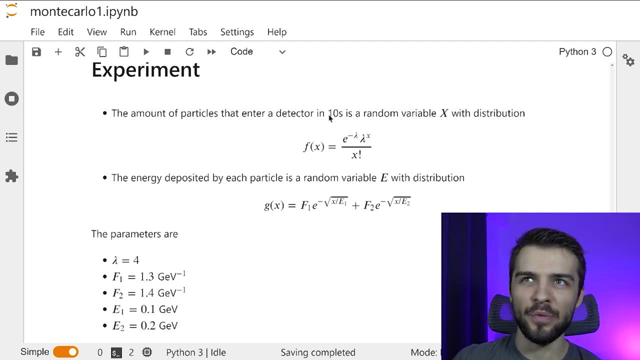 example, And hopefully that sort of makes you understand what this really means, And so let's sort of go over this. So suppose the amount of particles that enter a detector in a 10 second interval is a random variable, x with distribution, this, So it's a Poisson random variable. So I 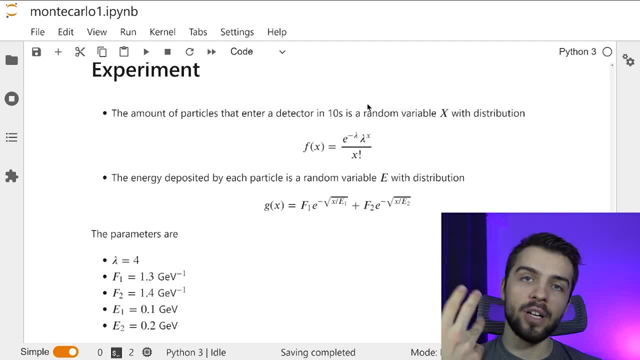 count for 10 seconds and maybe there's five particles one time, then I count for another 10, and then I count for another time and maybe there's 13.. So it's a distribution. So my experiment is counting the number of particles that enter the detector in 10 seconds. Well, that's one part. 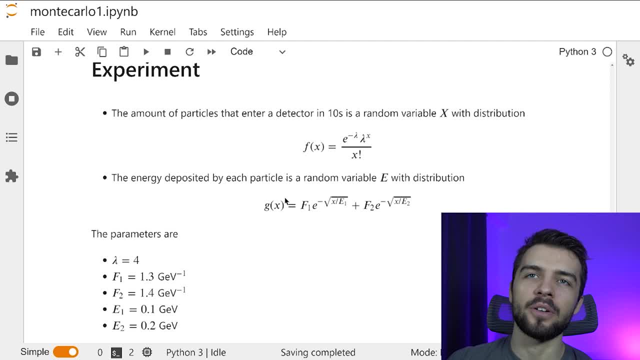 of the experiment. The energy deposited by each particle is a random variable, capital E, that has this distribution. So that's the distribution that I went over before. So there's a random number of particles being, you know, detected in the detector, But each one of those particles 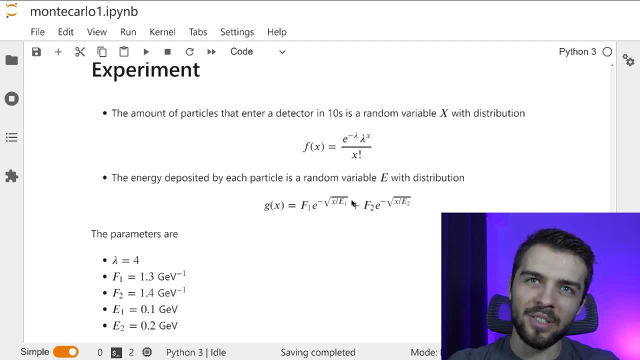 itself has a random energy. So you can see how things start to build up in these experiments, Right, And so what I'm interested in here is, in a 10 second interval, how much energy is deposited in the detector. So I have two random variables and I'll need to distribute, I need to sort of 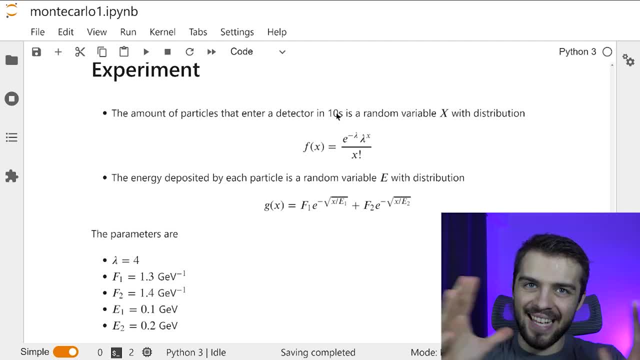 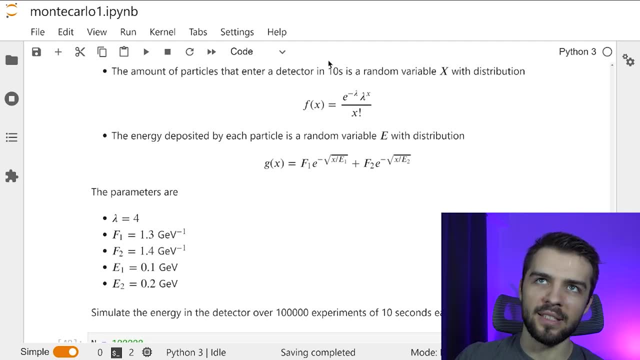 combine them together And then we can sort of simulate this 10 second of energy deposition in a detector cell. So the parameters here are: lambda equals four, That means the mean number of particles in 10 seconds is four particles. And then I have some values for F1 and E1 and E2 as 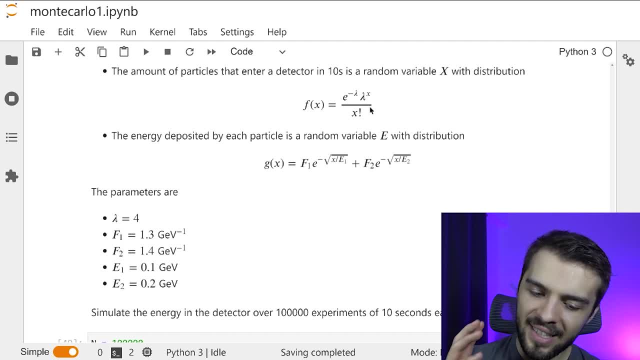 well here. So I know this distribution, I know this distribution. I know this distribution. Let's find out how much energy is deposited in a cell in 10 seconds. And you might wonder well, why are we interested in this? What's the point of this? And it could be that you're designing a 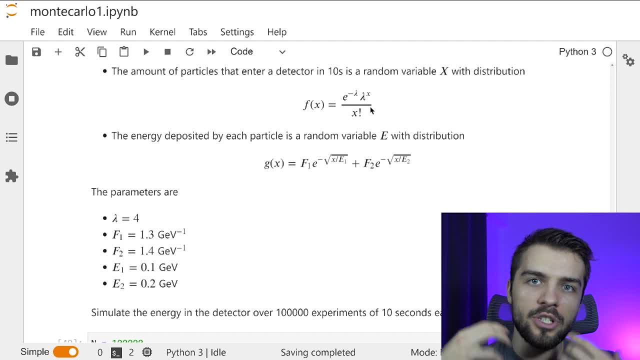 detector cell and you have to make sure that not too much energy is deposited or maybe it will break down or whatever. So these sorts of simulations are really useful And, believe me, it's all the time used in all experiments. In fact, the entire Atlas experiment has an entire 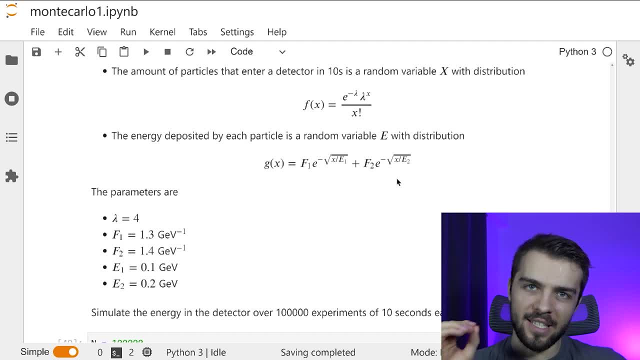 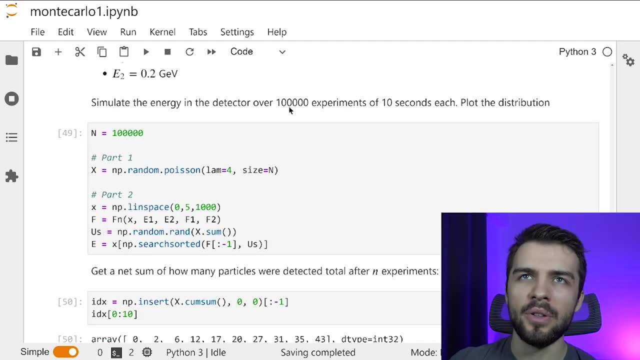 simulation side to it, just to check for things like this, to make sure that it's not just a random experiment, but to make sure that things will run well and that things agree with true experiment as well. So let's do 100,000 experiments of 10 seconds each. That'll give us a lot of 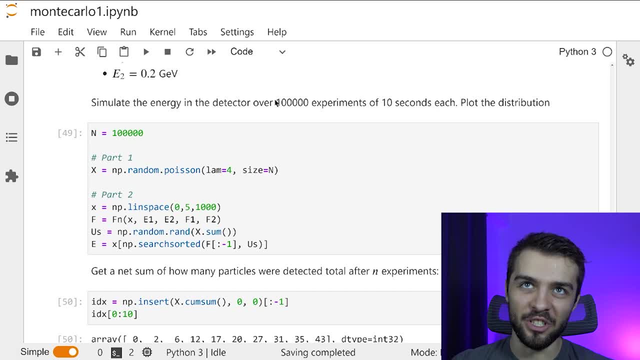 statistics Like, obviously, in real life you can't do this. And this is the nice thing about Monte Carlo is I can generate 100,000 experiments of 10 seconds each. So here n is 100,000.. I'm going to. 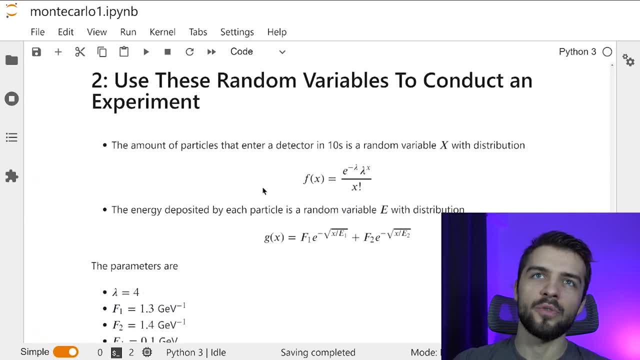 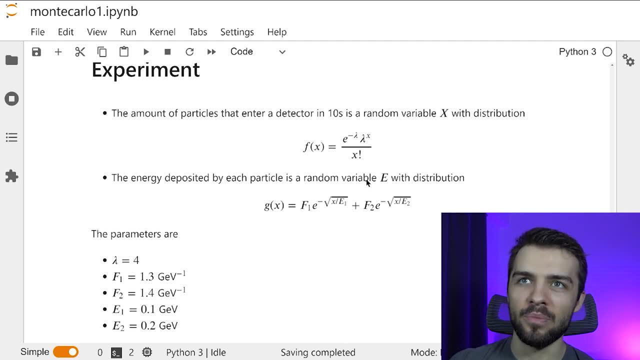 generate 100,000 Poisson variables with lambda equals four. So for each experiment that will tell me how many particles are detected in a 10 second period, Now I need also the random energy of these particles as well. So if there's maybe like 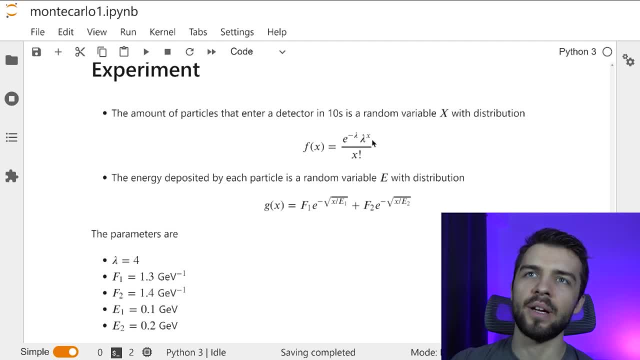 you know four particles and then three, and then eight, and then seven, and whatever. over 10 or over 100,000 experiments, there's going to be more than 100,000 particles detected. It's going to be the sum of all these. So I need to generate more energies, of course, than 100,000, because there's 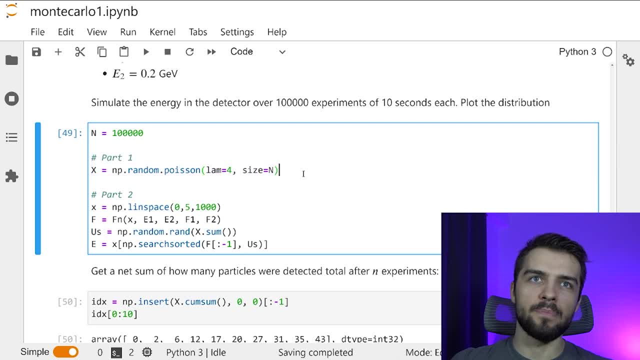 more particles than 100,000.. So this is part one, the Poisson, and part two is going to be the energies. So here I need to use my special way of inverting the function, which is what I do here, And the number. 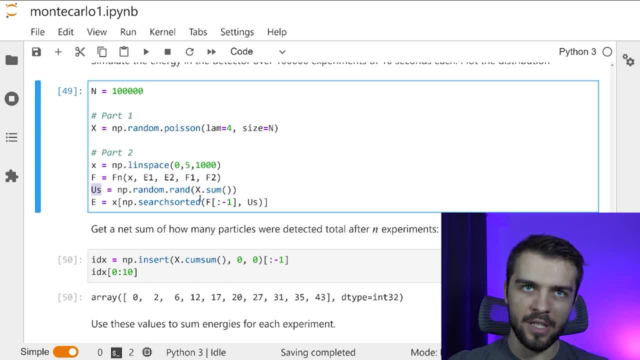 of use that I need. I need to generate- member- a bunch of different random energies is the sum of all the particles, which is just x dot sum. So I'm going to generate however many there is of this And then I'm getting my random energies using this inverse thing that I talked about in part. 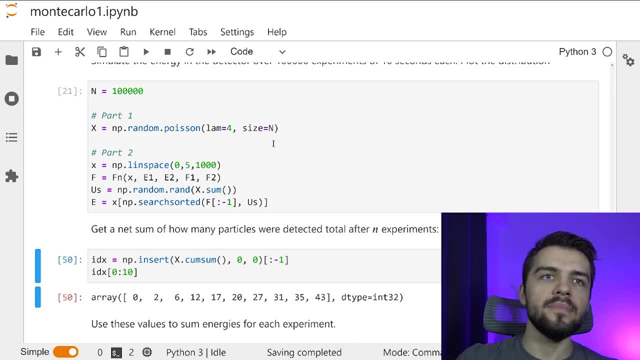 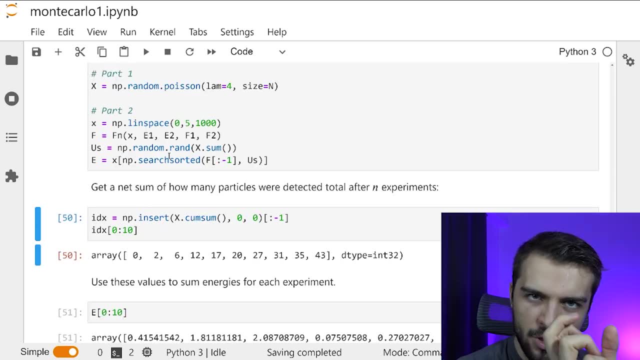 one of the experiment. So I run this, And so now we have all the random variables that we need. And so now for each experiment. remember the first experiment, maybe there was two detected. the next one, maybe three detected, then maybe five detected. we need to determine how much. 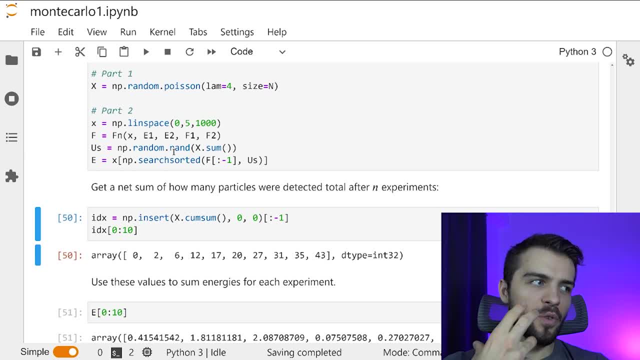 energy there was in each one of those experiments, And so there's lots of different ways that you can like loop over things and add up the energies and whatever, But I'm going to give you a kind of a clever way for how to do this. So the first thing I want to do in this clever way of doing 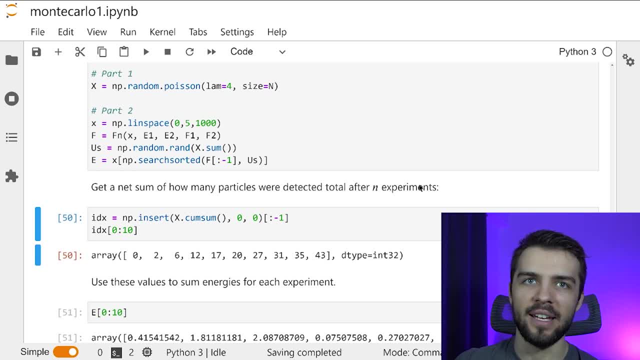 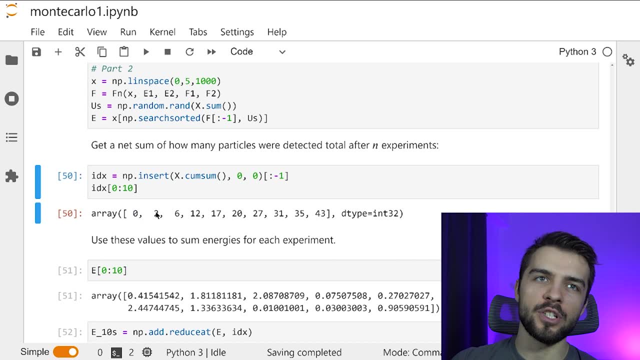 this is: we're going to get a net sum of how many particles were detected after n experiments And this is like a cumulative sum. So if I look here it says after zero experiments there were zero particles detected. After the first experiment there were two particles detected. 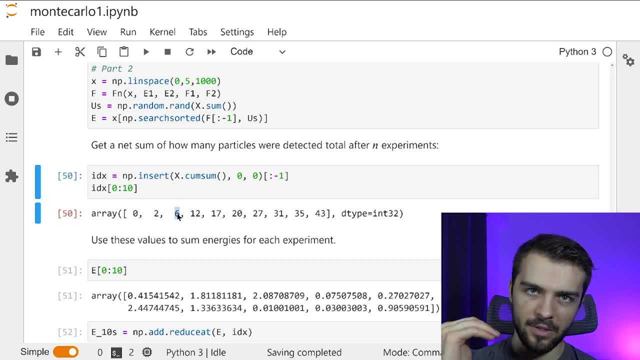 total. After the second experiment, there were six particles detected total three experiments, 1217.. So it's a cumulative sum of, after that many experiments, how many total particles have been detected. So then, what we can do is we can actually use these values here. to sum together: 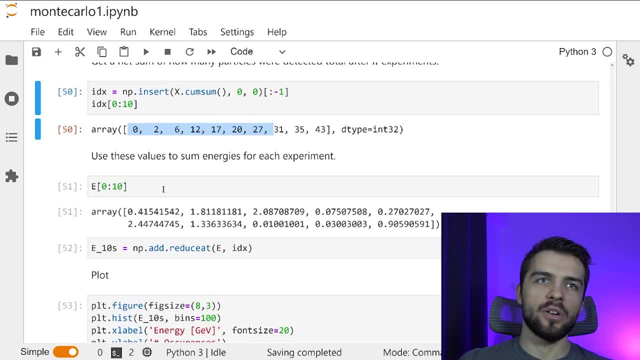 the energies over various experiments. right, And so these are the first 10 energy random variables that I have. But if I know that I have two particles detected in the after the first experiment, I would sum these two together and that would be the first experiment. Well, 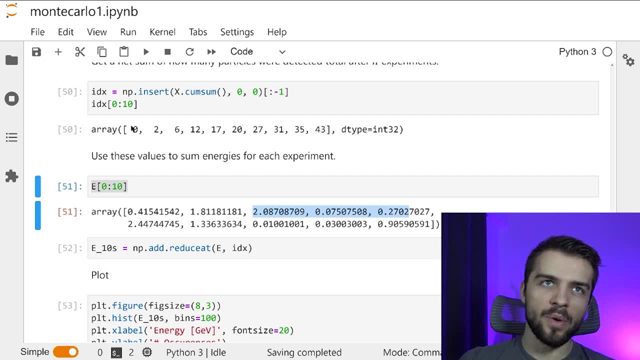 then six. right, I would need to sum the next four together, So I can use this array to say, all right. well, zero to two. I'm going to sum these two elements together: two to six. I'm going to sum the next four together: six to 12.. Well, I need to sum the next six together. 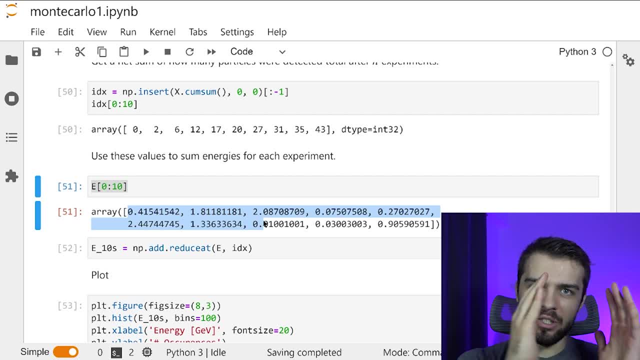 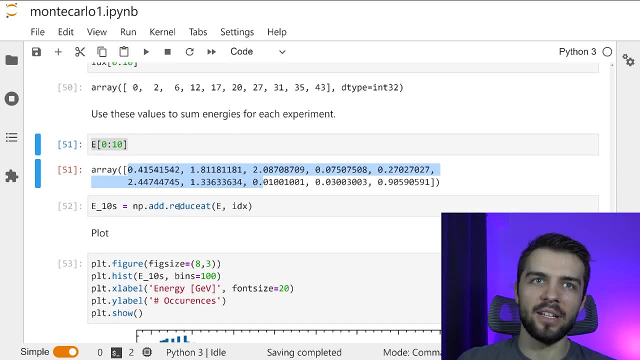 So I use this array and the array of energies to get the total energy for each experiment. Really think about that, because this is sort of tricky And I can use this np, dot, add, dot, reduce at with E and index, So it will sum. you know consecutive elements like this, So it'll sum. 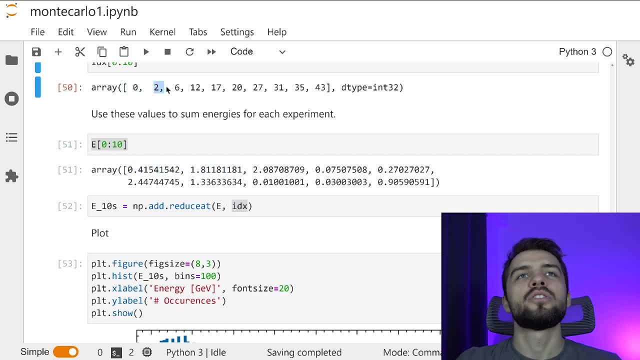 the zero to two. it'll sum these together. That's the first element of the new array. two to six: it will sum these four energies together. right, That's the second experiment. there were four energies And the elements in this array, this index that I generated here from x. 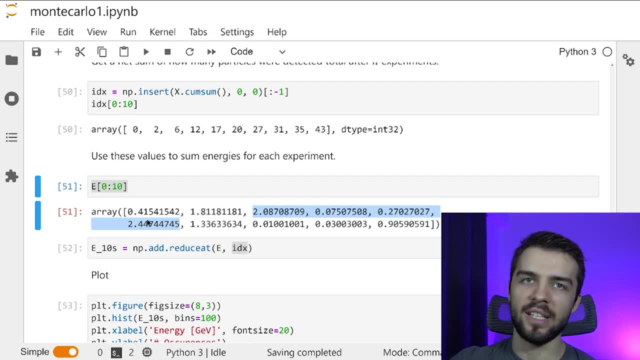 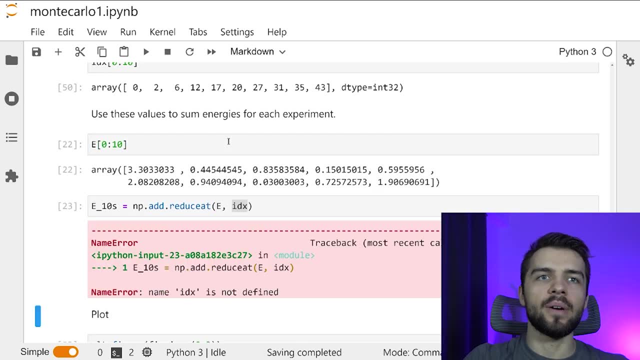 which is the number of particles, is the sum of these four energies And that gives the total energy, and then on and on. So that's what reduce at does in Python, in NumPy. So I can run this. let's actually run these first. So I have my indices, which is the trick, I have my energies. 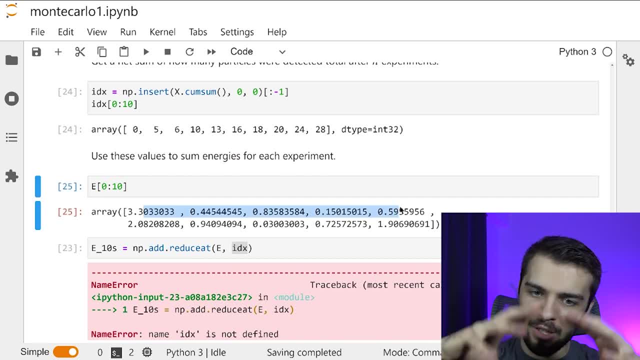 it will sum the first five energies together And that's my first experiment. the total energy for the first experiment. The next experiment, five to six. well, it's a cumulative sum, So there are only one particle detected in the next experiment. So the first experiment is all. 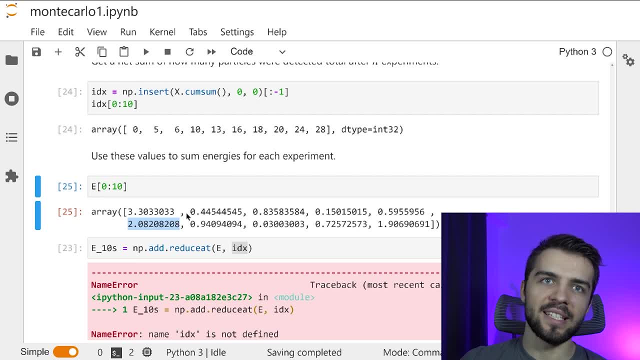 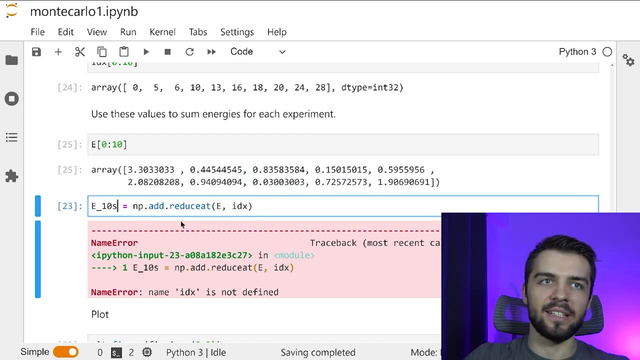 these energies. the second experiment will just be this energy and then six to 10.. Well, hopefully it makes sense. I've repeated it a few times now, So this is: gives me my E every 10 seconds. That's my array here. like this, Let's actually make sure it's doing what we want it to. 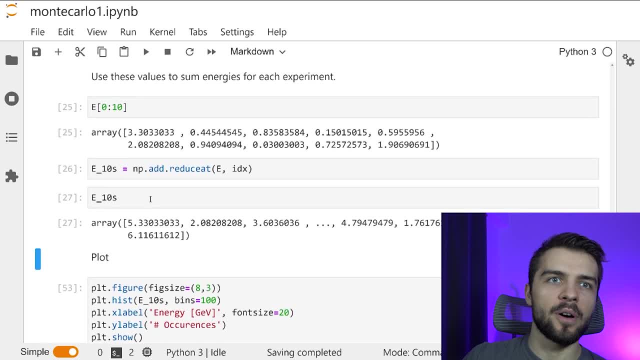 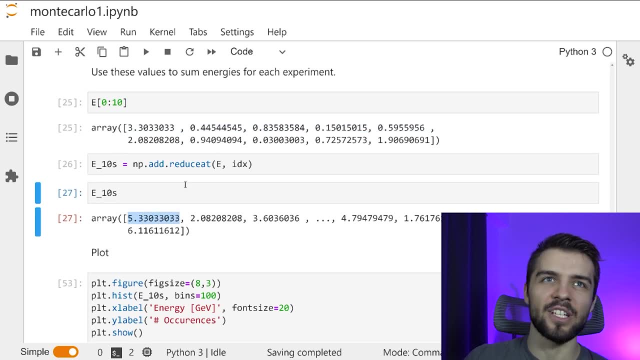 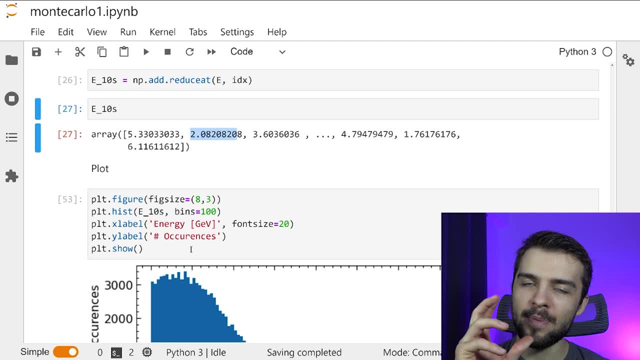 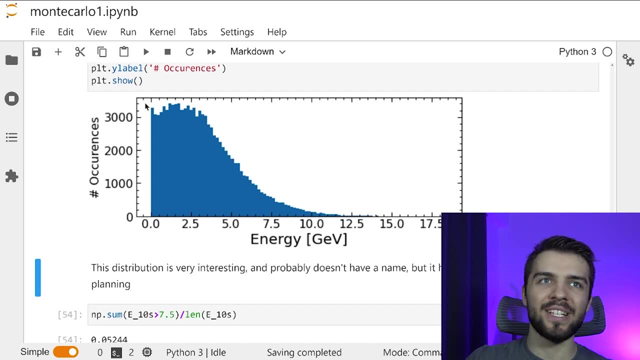 indeed, 2.08 is the energy that I get here. Now let's make sure. well, let's see what this looks like is what I plot here. So this is what the distribution of energy every 10 seconds looks like. this is a histogram, So you can see it's sort of flat here. So there's almost a flat region where 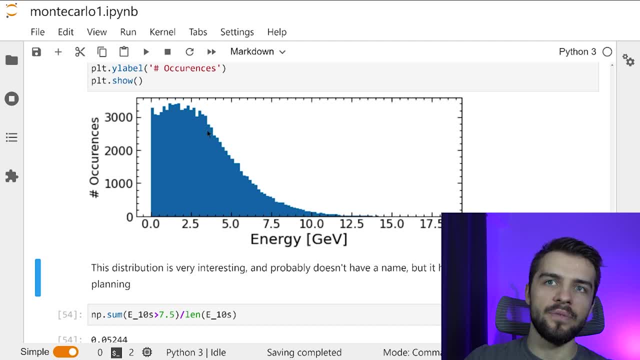 you know, a lot of these are between, maybe you know, zero to three GeV of energy, of particles, And then you sort of have this tail here. that goes like this: And so we've conducted an experiment, we've said we're going to look at every 10 seconds. our experiment is 10 seconds. 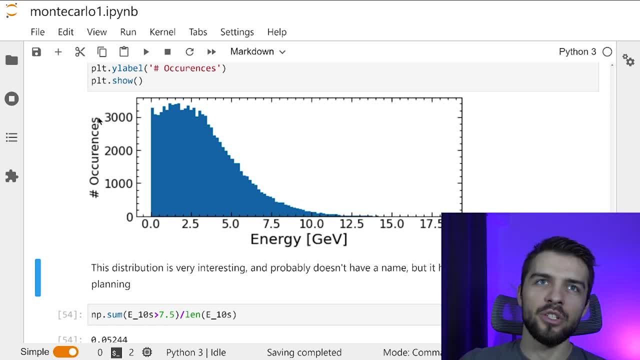 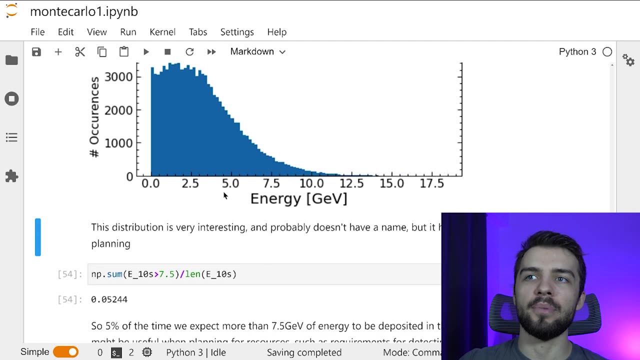 how much energy is deposited in the detector, And we get this looking distribution that probably doesn't have an explicit formula for it, Or, if it does, it's probably very complicated. So we have a distribution that looks like this. Now, having run that Monte Carlo, we can then, you know, determine interesting things, for example, 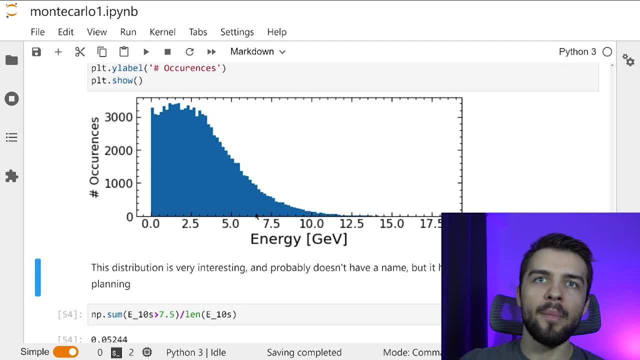 right. So, for example, let's look at how much of this histogram is, you know, above 7.5 GeV of energy, because maybe we really don't want high energy deposited in a detector cell every 10 seconds because the detector maybe there's a certain amount of material that can be ionized. 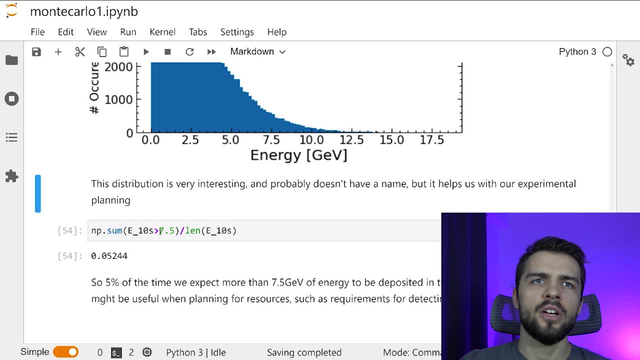 and it needs to refresh or whatever, so you can't have too much energy. So if I look at the proportion, like how much you know is in this region, you know- I'm just summing up- you know how much of these are greater than 7.5 divided by the total number of events And you can see. 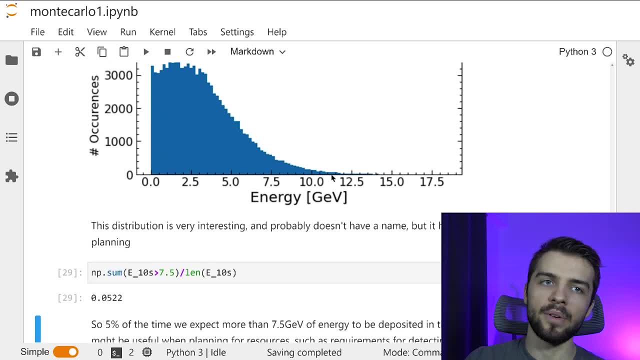 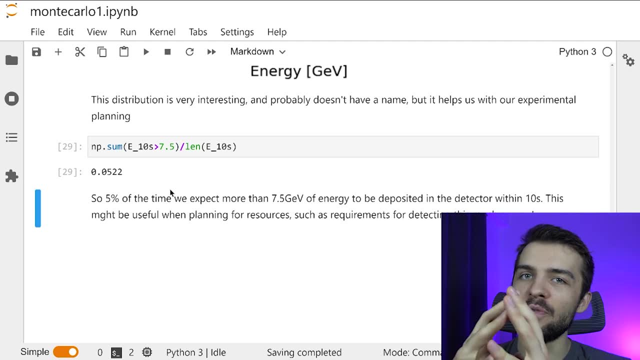 that is about 5.22% of things that are above 7.5.. So what it means is that 5% of the time we expect more than 7.5 GeV of energy, And this could be useful when actually planning, like the. 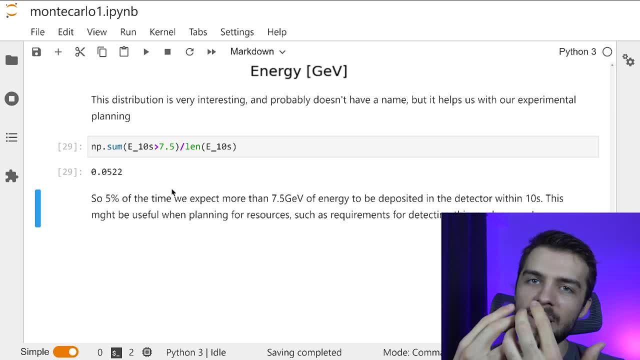 materials you need for the detector, what it sort of needs to compensate for, and all things like that. So this is a little bit of a taste of what Monte Carlo is and really how it can be useful in experimental planning And in the Atlas experiment. 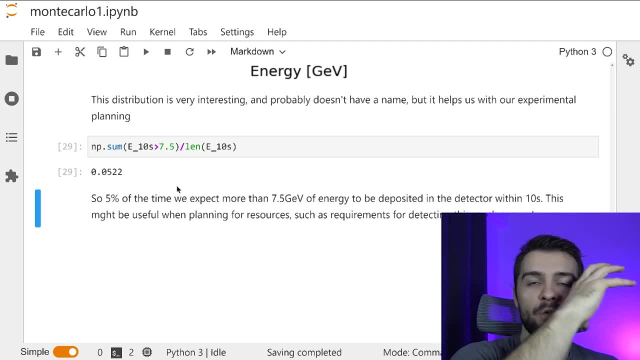 like I said, they have an entire simulation and then the entire physical experiment, and they'll actually compare the results of the two to determine things like new particles, for example. Anyways, I hope this video was useful. Be sure to check out all my other videos. 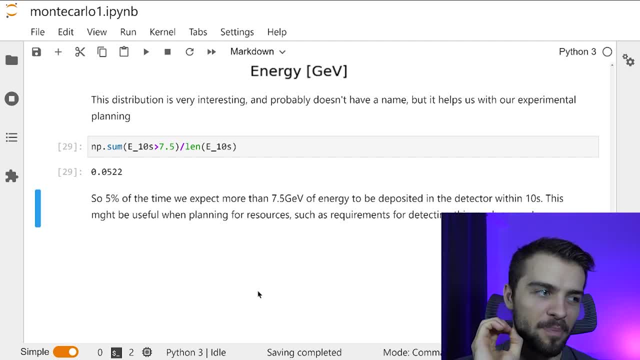 as well. There might be a short video in the future about how to compute pi- the actual value of pi- in Python, using no beforehand knowledge of pi, just using random variables. Anyways, thanks for watching and I'll see you next time.